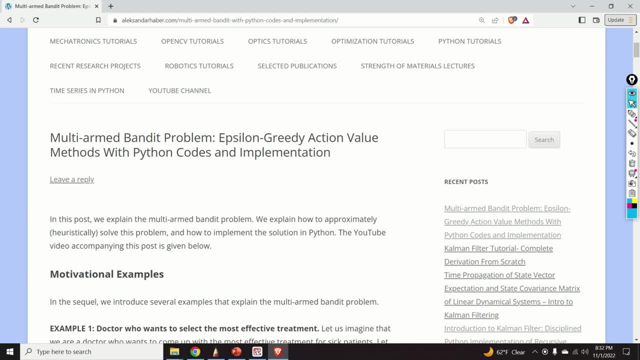 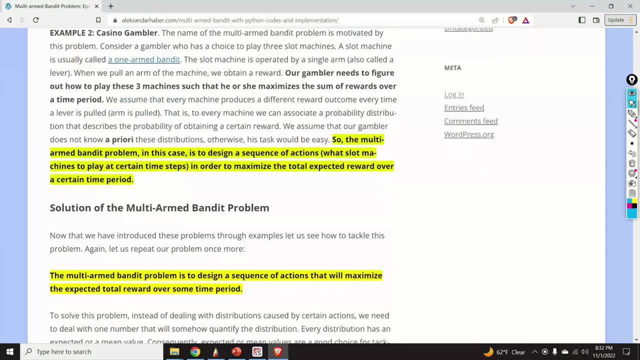 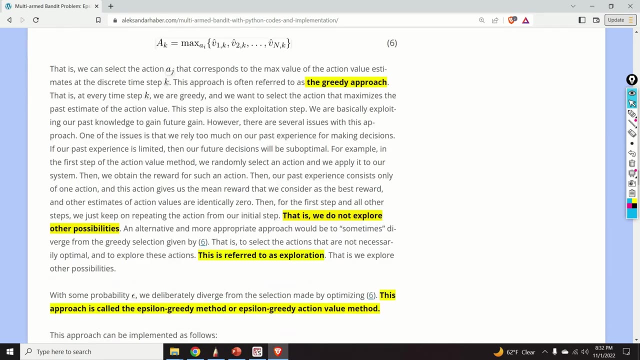 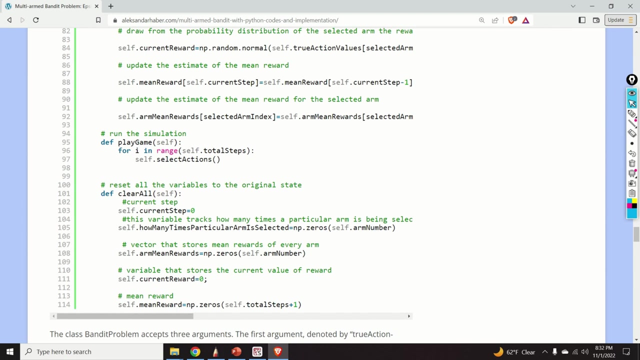 that I will explain in this video, And here is the post. The post contains motivational examples, contains graphs, equations, explanation of all the equations and, finally, it also contains Python codes. A link to this post is given in the description below this video. Before: 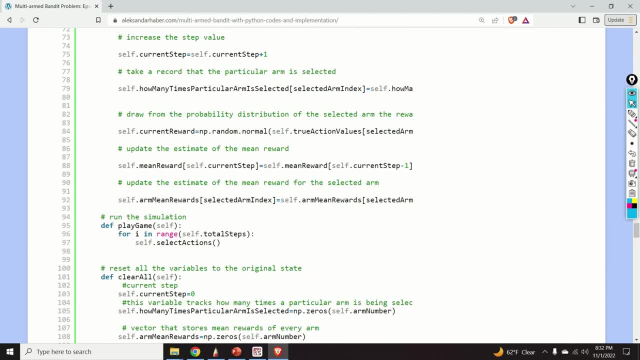 I start, I would also like to mention the following: It took me a significant amount of time, energy and effort to create this video and the accompanying post. Consequently, I kindly ask you to press the like and subscribe buttons. Thank you very much. 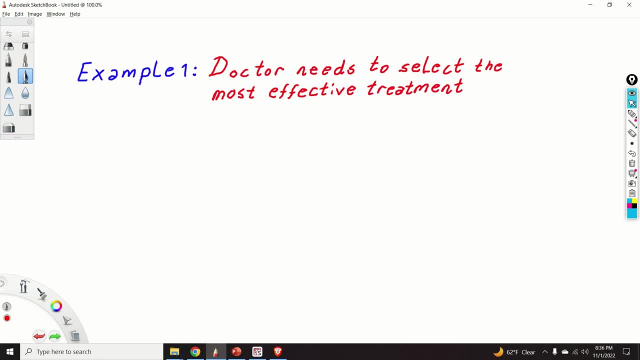 Okay, so let's start with motivational examples. The first example is the example of the doctor who needs to select the most effective treatment for his sick patients. Now, let us assume that we are a doctor and this is us. We are a doctor. And, in addition, let us assume: 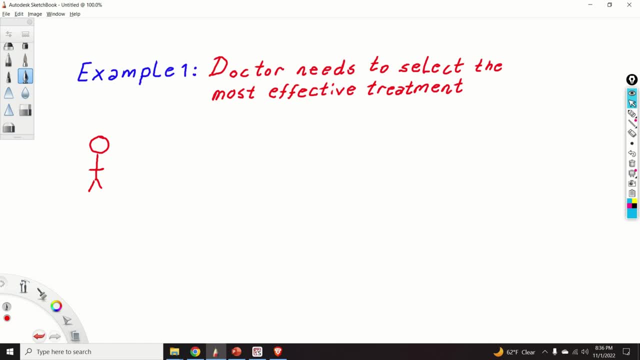 that we have three possible treatments that we can select And let these treatments be called actions. So this is our first treatment, This is action one, Then we have the second treatment, This is the action two, And then we have the third treatment, and this is the. 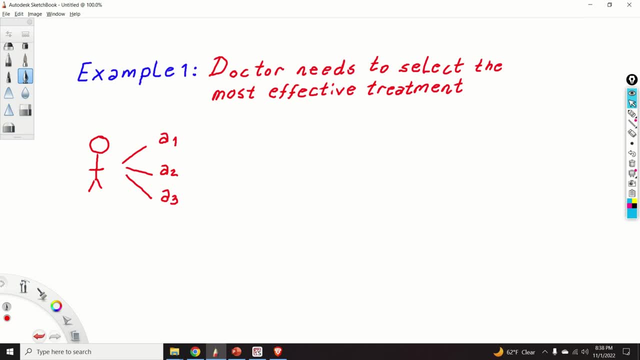 action number three. Next, let us assume that every time we apply the same treatment or action, we obtain a different health outcome quantified by numerical value. The health outcome can be, for example, the percentage of the recovery of the patient from the disease, or some numerical measure. 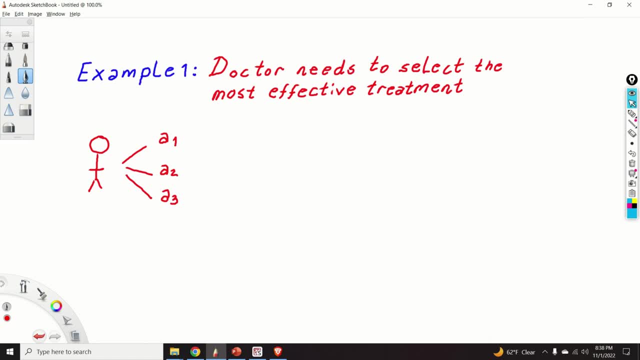 that measures the presence of a virus or cancer in the body of the patient. The variability of the same outcome can be due to the number of patients, So let us assume that we can to the many factors. for example, every patient is different and every person will most likely. 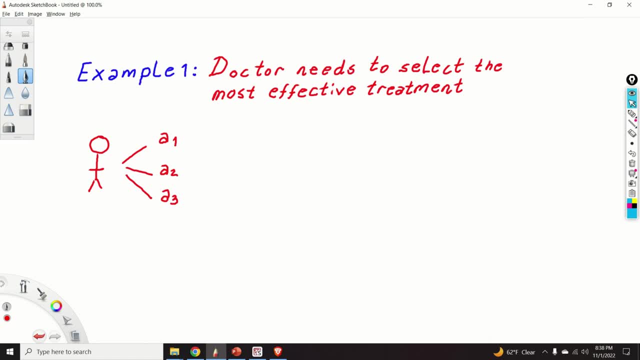 react differently, even slightly, to the same treatment. even we apply the same treatment or action to the same patient over a time interval, we will most likely obtain different results. if we would have enough data, that is, past data, of applying different actions and measuring the patient outcomes, the recovery outcomes, then for every action we can actually construct 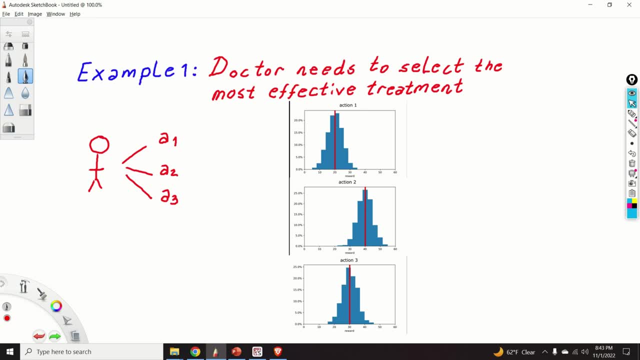 a probability distribution that can quantify the effectiveness of the treatment or of the action. now we call the numerical value of the outcome as the reward. more positive, the outcome that is more positive, the reward that is, if you measure the percentage of the recovery of the patient, let's say in 10, 30, 40, then this percentage value can be our reward and we want to basically 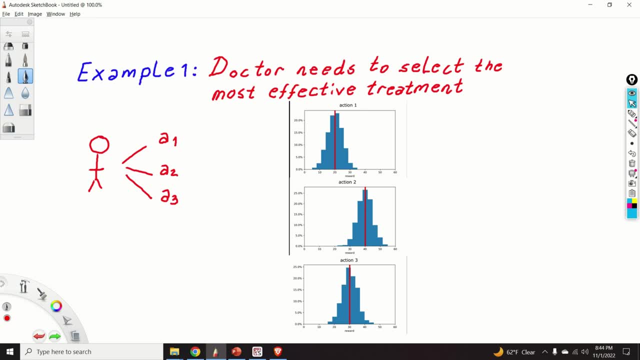 maximize this reward. again, the higher the reward, the more effective the treatment is for a particular patient. again, assuming that we have enough data, we can construct the probability distributions that you can see over here. so, for example, this graph over here shows the distribution of the rewards for the action a1 and we can observe here that the mean is equal to 20.. 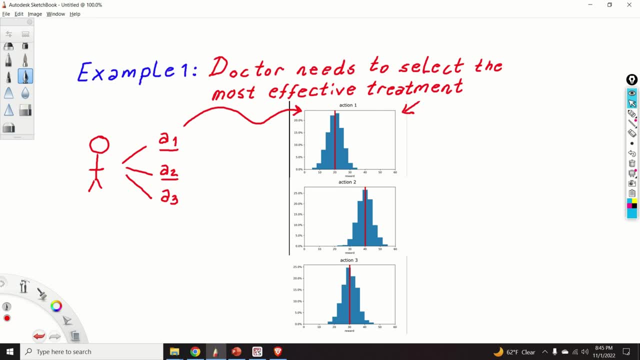 for the treatment a2 of or for the action a2. this is the probability distribution with the mean, let's say, of 40. and for the action number three or for a3, we have the probability distribution of rewards that's given over here. so assuming that we know these distributions, then our 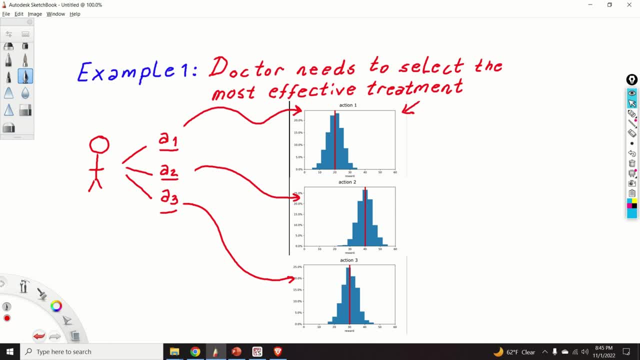 sum of exactly this, the combination of theYa search result over here, and then we leave it for 1, and now the answer is 2, 1, 3, 4, and so this is the second看 یہ, the women's, the patients. we can see here that the mean is 40, so the mean of reward is 40. 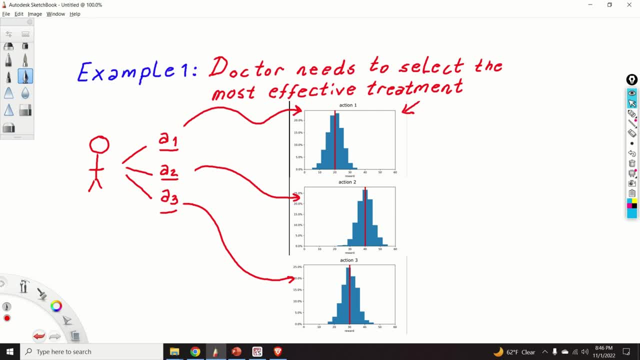 so by applying this action we can get most likely outcome of basically of reward to be around 40 and you can see how the means for other actions are kind of like shifted left to. this mean. so if we continuously apply the action a to, we can hope that we can get the best results. that is, we can hope that 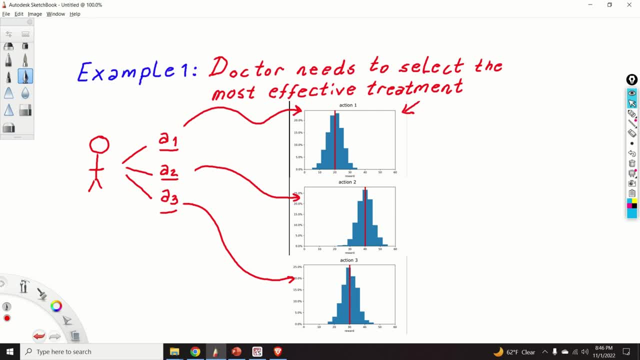 patients will more positively react to this treatment compared to this treatment or the action one treatment. however, there is one big catch here: we don't know these distributions are free, or so when, say, let's say, pharmaceutical company start to design these actions- actions they don't have past data they don't have. usually they don't have and they have to do. 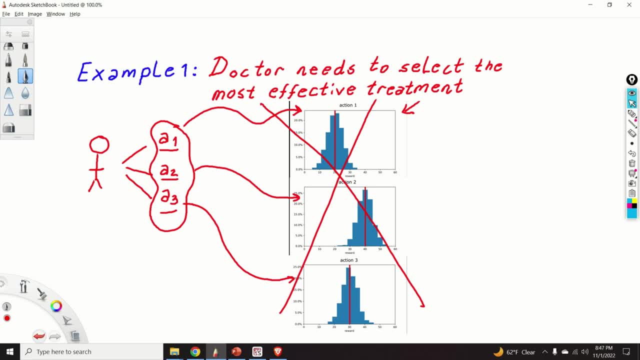 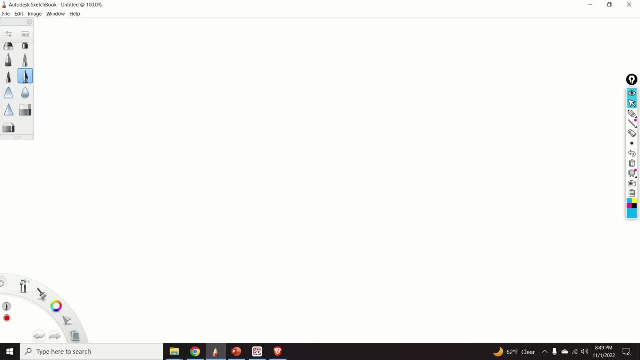 clinical trials and other experiments. the multi-armed bandit problem is to design a sequence of actions that will maximize the expected total reward over some time period. also in the literature, this problem is defined as the problem that ends up finding a sequence of actions that will maximize the sum of rewards over a certain time period. okay, so the idea goes like: 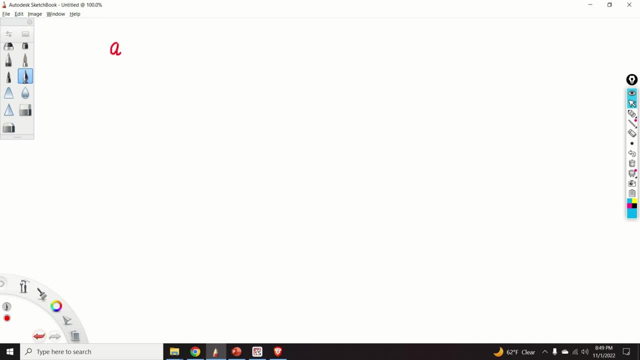 this. let us say that we have three possible actions: a1, a2 and a3. now, at the time, step k is equal to 1. since we don't have any data, we need to randomly choose an action so we can say that our action A1 is equal to, let's say, A3. this subscript here denotes: 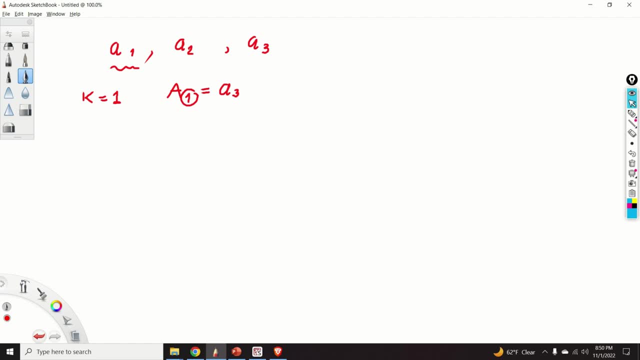 the discrete time instance 1 and over here the lowercase letters are possible actions and this action will produce certain data reward, Let's say reward R1.. Going back to our example of a doctor, that who wants to design a treatment for patients. basically, doctor randomly chooses an. 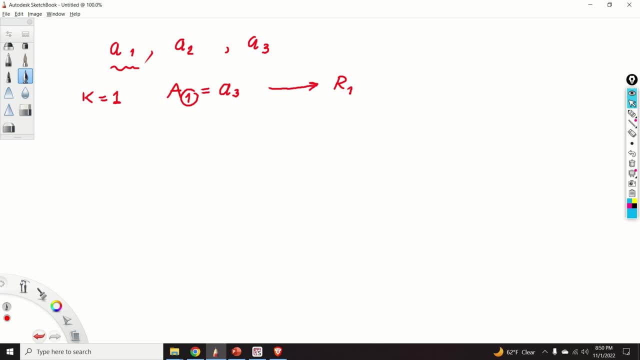 action finds a patient, applies that action, observed the health outcome and records that health outcome. Now the main question is how to select an action for the time step 2,, that is, what will be our a2.. Will it be a1,, will it be a2, or 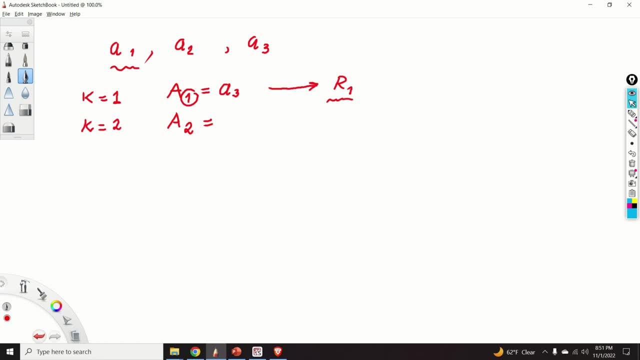 will it be a3,? when I mention a1 and a2 and three, I mean lowercase letters. that is the actions. So at time, step 2, we either pick up another patient or same patient after some time interval and we need to somehow figure out how to determine the proper actions on the basis of our past. 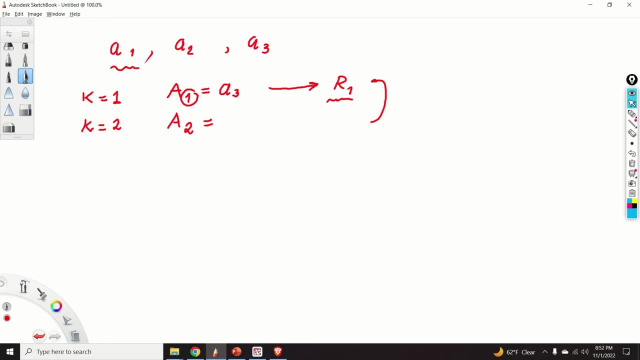 experience. and here the experience is very limited, since we have only tested the action A3.. The multi-armed bandit problem aims at finding the sequence of actions that will maximize the sum of rewards over a certain time period. So let us say that at the time step k is equal to 2, capital A2 is equal. 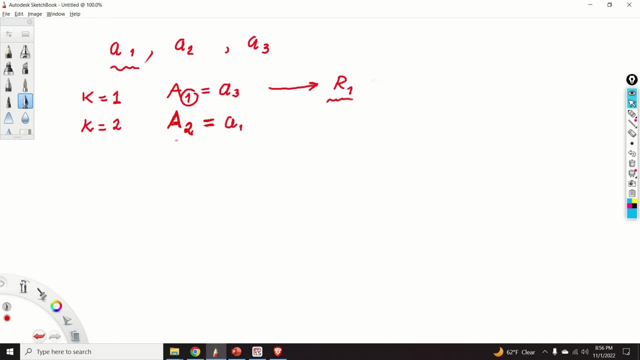 to action A1 and this action produces the reward R2.. Then at time step k is equal to 3, capital A3 is equal to R2.. a1, that is at a time step 3. we select action 1 and this action produces reward. 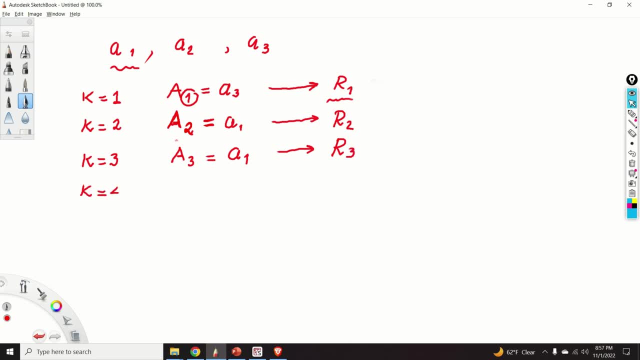 r3, then at the time step k is equal to 4, our action is equal to action 2 and this action produces the reward r4. so the multi-armed banded problem ends at finding a sequence of actions that will maximize the sum of rewards over a time period. so if we continue this, 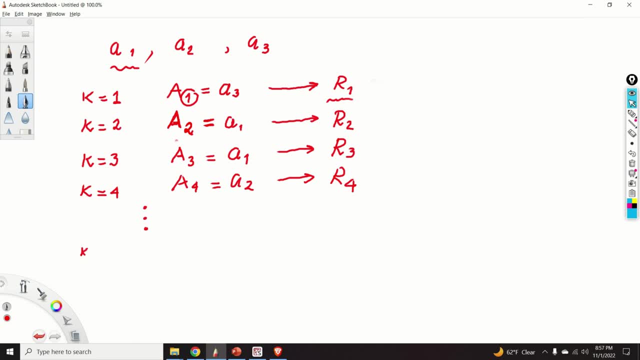 process over, let's say, n steps. the solution of the multi-armed banded problem will minimize this sum r1, r1 plus r2 plus r3 plus r4, until rn again. as i mentioned previously, in the literature this problem is also defined as maximizing the expected total reward over some time period. 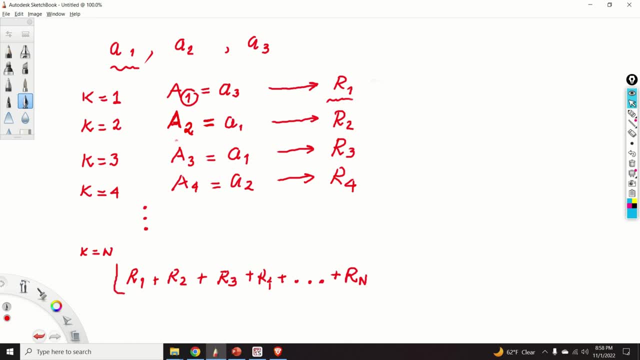 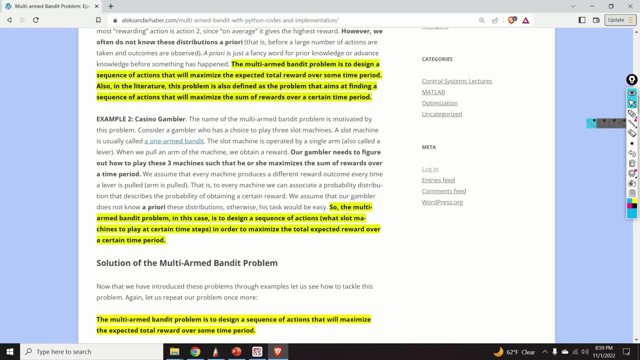 so you can, instead of minimizing or actually maximizing this quantity over here- and let's call this quantity r sum n- an equivalent problem would be to minimize r sum n divided by n. okay, so this was our first motivational example, so let us briefly go over the second motivational. 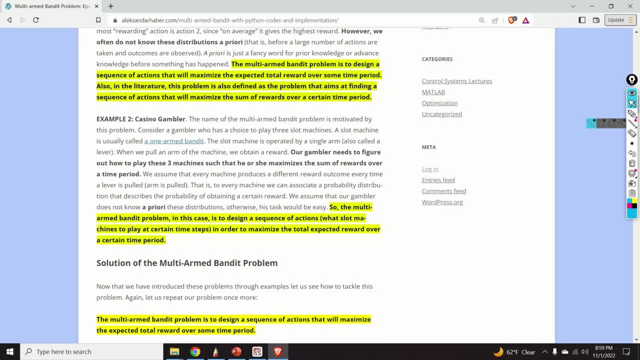 example, and that example is called casino gambler. okay, so this is our first motivational example, so let us briefly go over the second motivational. The name of the multi-armed bandit problem is motivated by this problem. Consider a gambler who has a choice to play three slot machines. 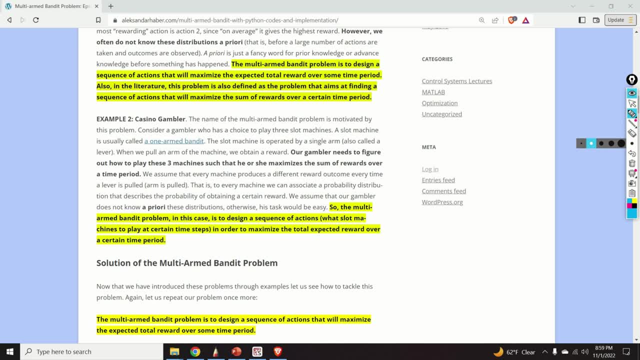 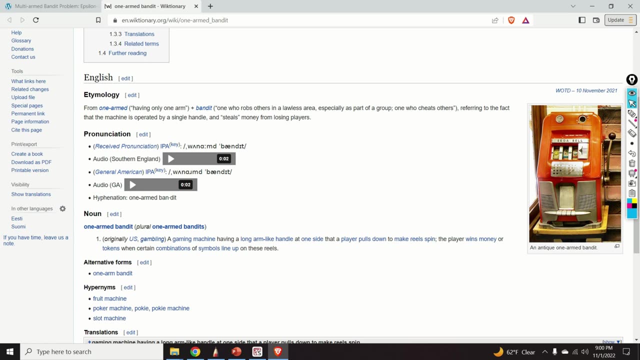 So we are having a gambler in Las Vegas and he can play three slot machines. A slot machine is usually called a one-armed bandit And you can see a Wikipedia page over here that shows you an old or vintage one-armed bandit. 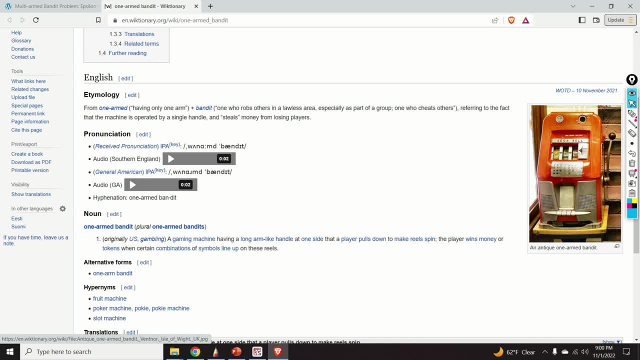 So this is a quite old machine, maybe 60-70 years ago. You basically pull this arm and you get some combination of fruits, And this combination of fruits gives you some points, or gives you money, Or you lose money, depending on what you do. 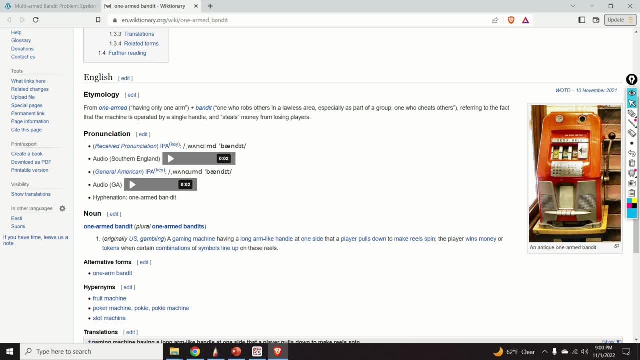 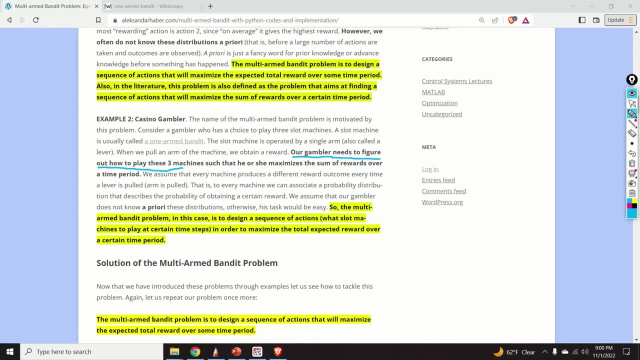 Usually you lose money in casinos. Now our gambler needs to figure out how to play, let's say, three machines we have such that he or she maximizes the sum of rewards over time period. So we are playing the game and we hope that over time our profit will increase. 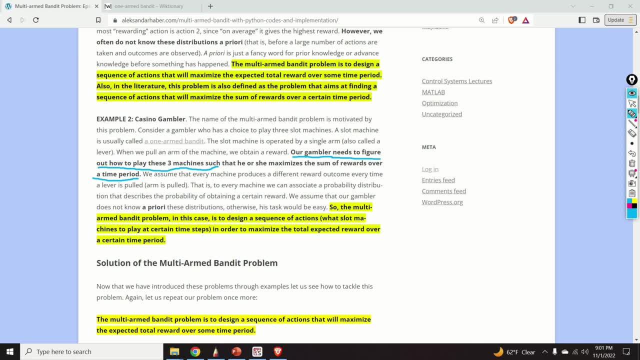 Now we assume that every machine produces a different reward outcome every time a lever is pulled or arm is pulled. That is, to every machine we can again associate a probability distribution that describes the probability of obtaining a certain reward. We assume that our gambler does not know a priori these distributions. 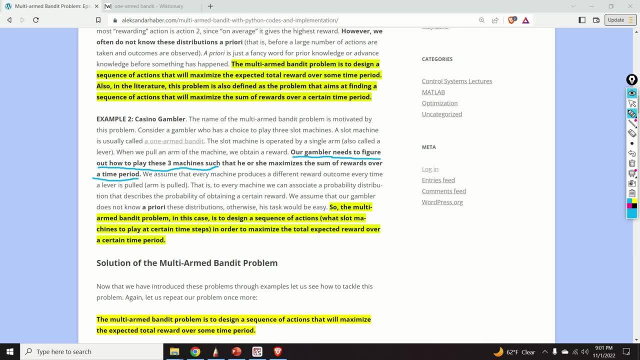 Otherwise his task would be easy. He would take or he would play the machine that has the most favorable outcome, That is, the machine for which the expected value of the outcome is the largest. So the multi-armed bandit problem in this case is again: 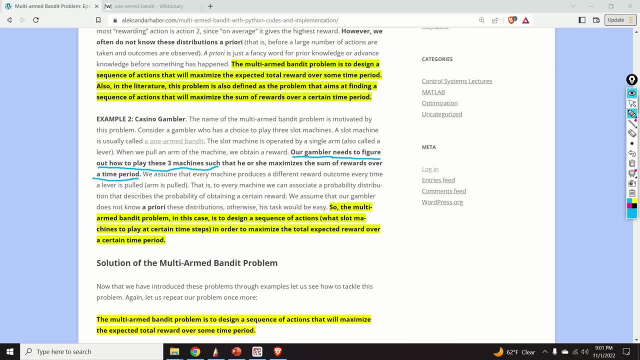 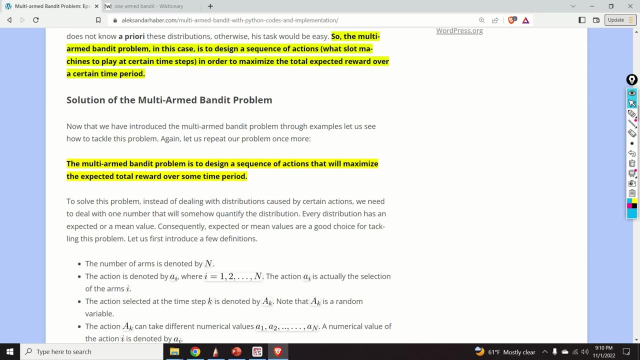 to design a sequence of actions- what slot machines to play at certain time steps in order to maximize the total expected reward over a certain time period. Now that we have introduced the multi-armed bandit problem by using several examples, let us see how to tackle this problem. 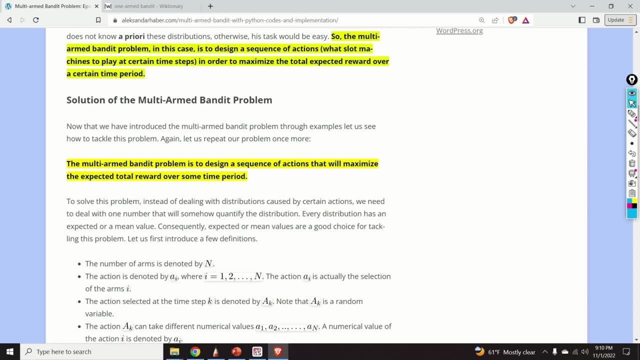 However, let us repeat our problem once more. I am doing this because I am following advice of old latins. So there is an old latin proverb saying repetition is mother of knowledge. So the multi-armed bandit problem is to design a sequence of actions. 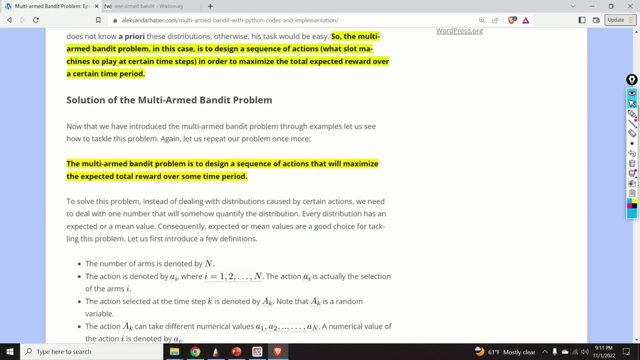 that will maximize the expected total reward over some time period. To solve this problem, instead of dealing with distributions caused by certain actions, we need to deal with one number that will somehow quantify the distribution To explain this, so let us illustrate a typical, normal Gaussian distribution. 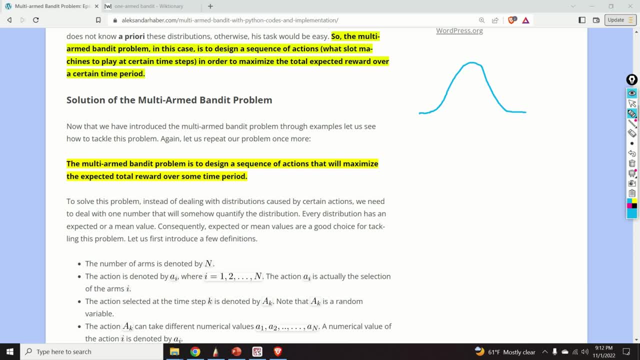 So it is very difficult to deal with distributions, although there are some statistical methods to deal with distributions. instead of dealing with distributions, we can somehow deal or compress this distribution to a single number, and that can be the expectation or the mean value of this distribution, and let this be, let us say, a mean reward. 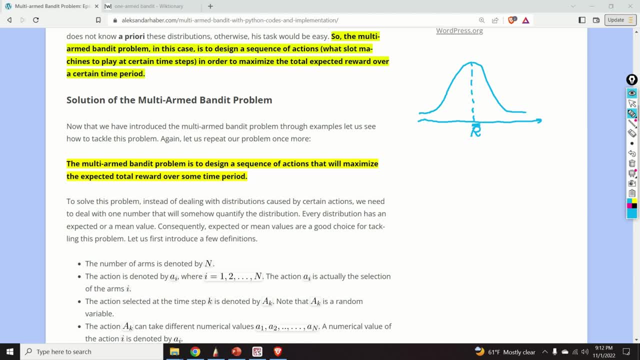 Now we are using the expected value or mean values, and there are good choices I mentioned, for tackling this problem. However, before explaining how to tackle this problem, let us introduce a few definitions. The number of arms is denoted by n, So we have n arms and we need to find a way. 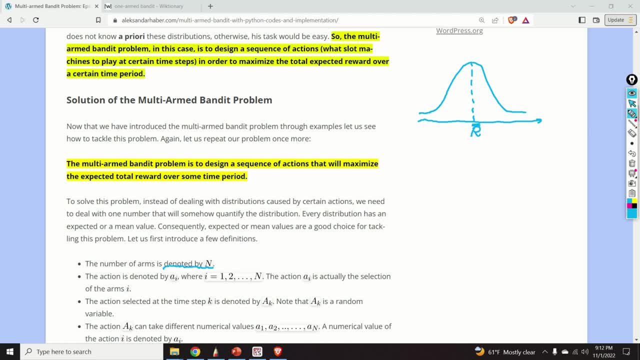 how to properly choose them over time in order to maximize the expected total reward over some time period. Then the action is denoted by ai, where i can go from 1 to n. The action ai is actually the selection of one of the arms. i. 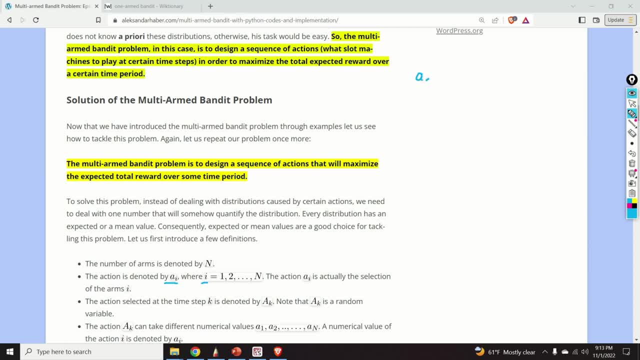 So let us say that we have three actions: a1,, a2, and a3.. This action a1, will produce a probability distribution of rewards that will look like this: The action a2 can produce a probability distribution that can, for example: 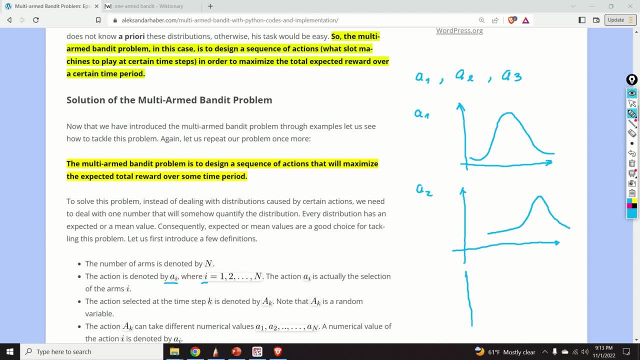 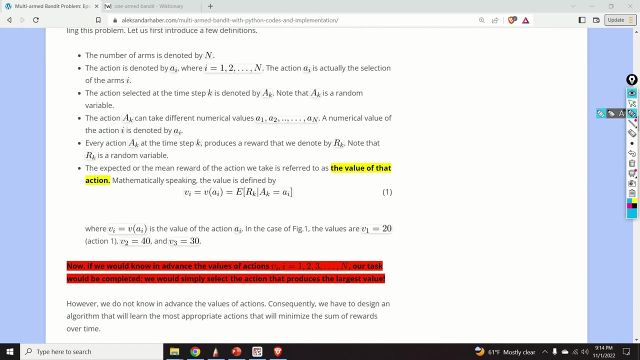 look like this, And the action a3 can produce the probability distribution of rewards that can look like this. The action selected at the time, step k, is denoted by aK and know that aK is a random variable. What does this mean? 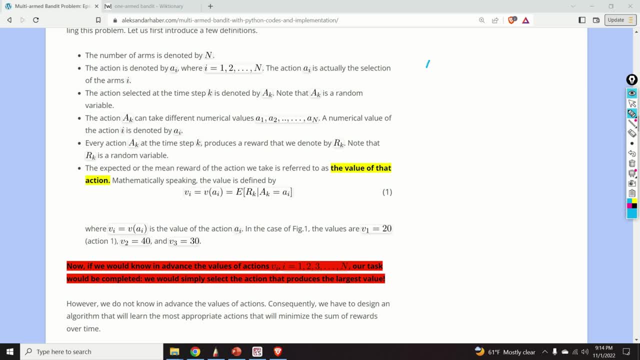 It means the following: If, at the time step k1, we basically select action a1, capital A1, to be equal to action 1, then the reward will be r1.. Now let us say that at the time step k2, we select a2 to be a1.. 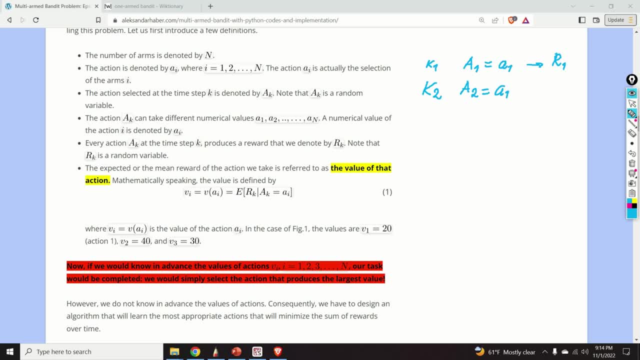 So again, what happens is that we select the same action. However, this does not mean that action at the time step 2 will produce the same reward as in the step. k is equal to 1. That is, r1 is not necessarily equal to r2. 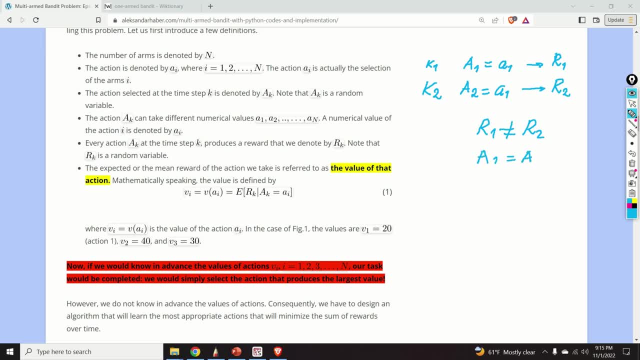 although a1 is equal to a2.. This is because we are dealing with distribution. So if this is a distribution for a1, and these are the rewards at every time step, we are basically randomly selecting a value. So if we select a1, 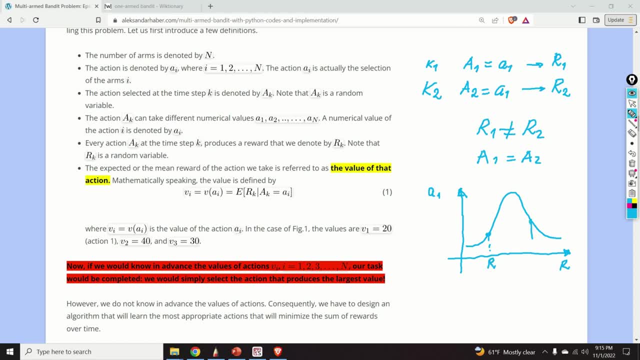 the reward can sometimes be here, or the rewards can be here, but most likely they will basically be around this region. Okay, the action ak can take different numerical values. can take a1, a2, up to an A numerical value of the action. i. 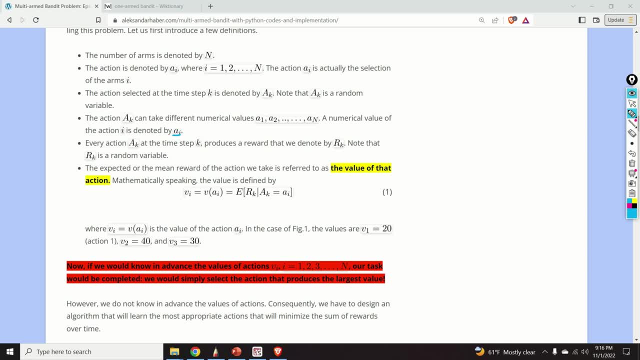 again, is denoted by its lower case, ai. Every action ak, at the time step k, produces a reward that we denote, as explained previously, by rk. Note that rk, as explained previously, is a random variable, The expected or the mean reward of the action we take. 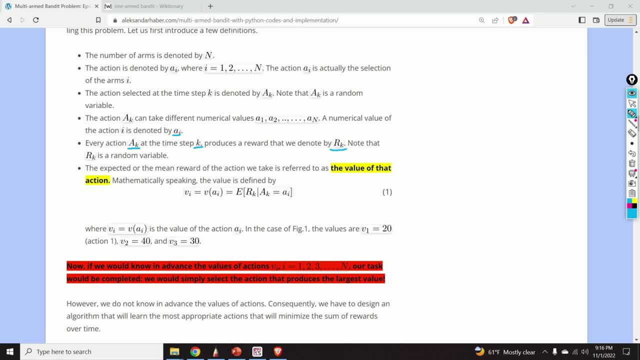 is referred to as the value of that action. So this is very important to understand. The expected or the mean reward of the action we take is referred to as the value of that action And mathematically speaking, the value is defined as: 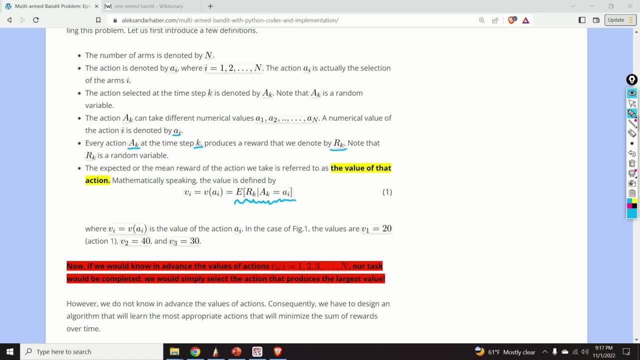 the expectation over rk, over the rewards, when the action is equal to ai. So what happens over here? We basically have ai, action and its corresponding distribution of rewards. The expected value of this distribution of rewards for the action, ai, is actually our vi. 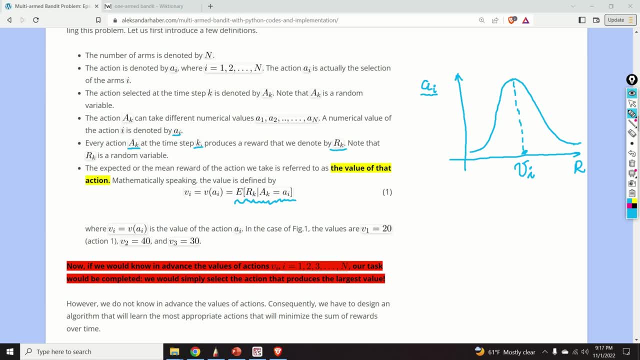 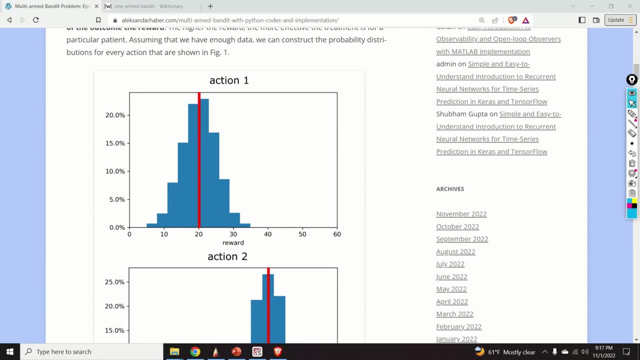 and that is our action value, The value of that action better to say. Now let us go back to our figure 1 from the beginning of this post and let us see what are the values of actions. So here for the action number 1. 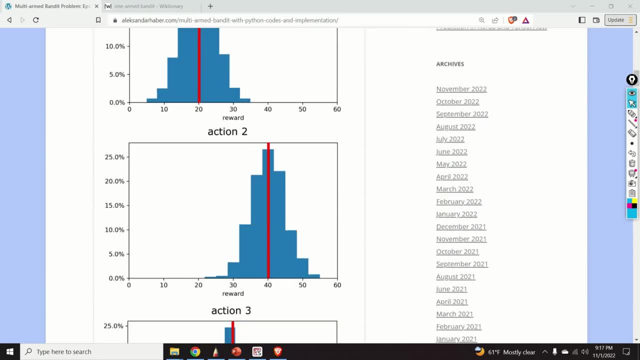 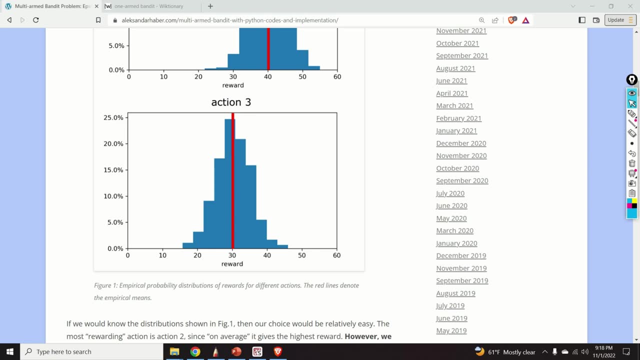 the value of the action is 20.. For the action number 2, the value of the action is 40 and for the action number 3, the value of the action is 30. Now you can see over here that I have one very important comment. 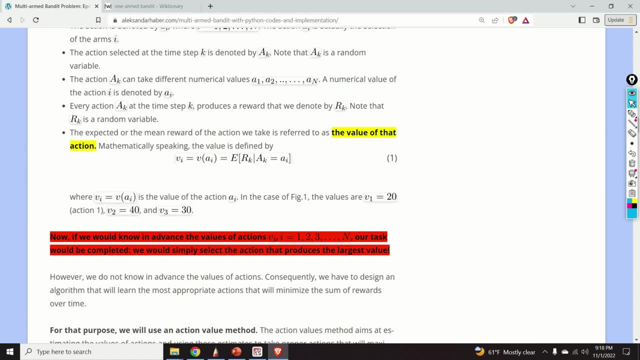 that I marked in red, And this is very important to remember. If we would know in advance the values of actions v1,, v2, v3 up to vn, our task would be completed. We would simply select the action that produces the largest value. 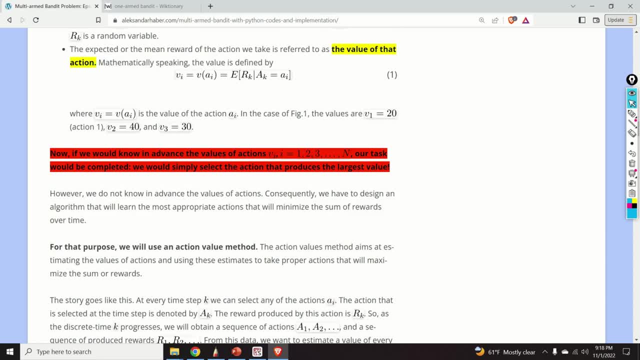 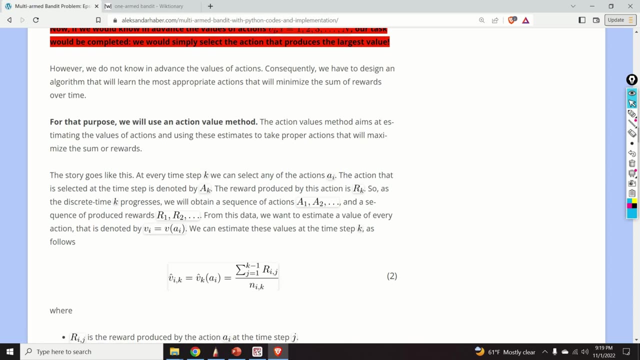 However, we do not know in advance the values of actions. Consequently, we have to design an algorithm that will learn the most appropriate actions, that will minimize the sum of rewards over time, And for that purpose we will use the action value method. 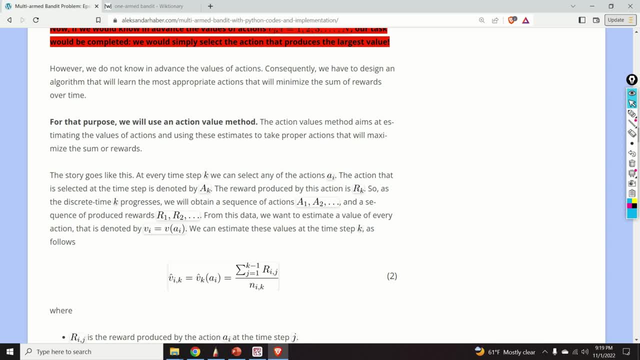 The action values method aims at estimating the values of actions and using these estimates to take proper actions that will maximize the sum of rewards. So the story goes like this: At every time step, we can select any of the actions Ai The action that is selected. 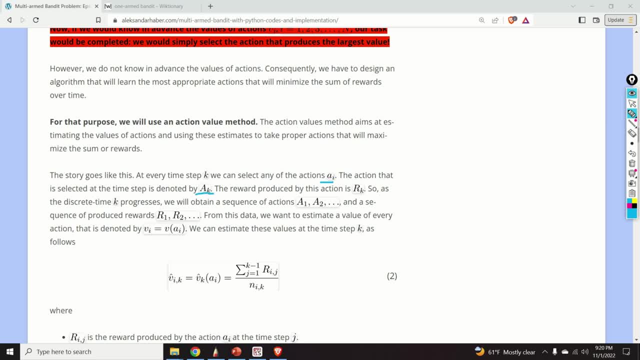 at the time step is denoted by capital Ak. The reward produced by this action is Rk. So as the discrete time k progresses, we will obtain a sequence of actions a1, a2, etc. and a sequence that produces rewards r1,, r2, etc. 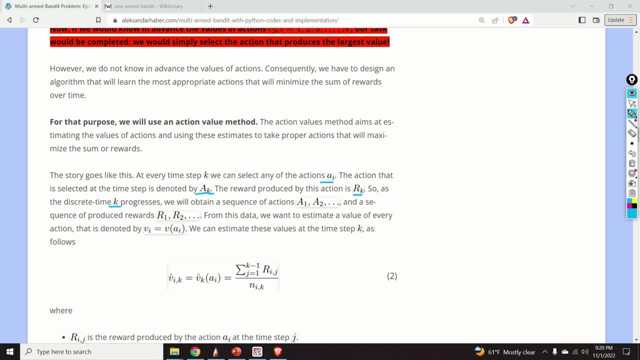 From this data, we want to estimate a value of every action that is denoted by Vi and that is equal to V. Now we can estimate these values at the time, step k, as follows. So here is the formula for estimating the values, the actions. 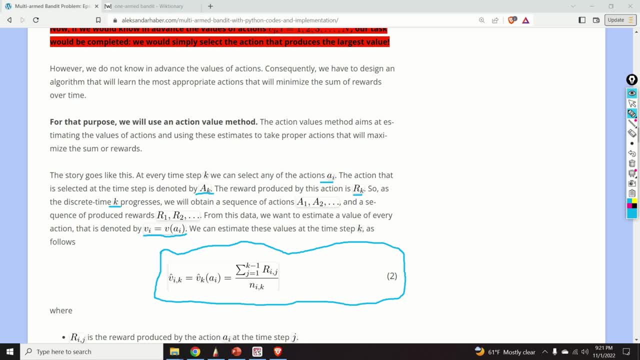 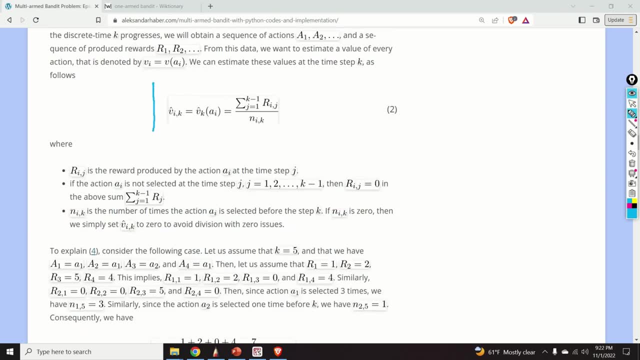 the values of actions at the time, step k. So let us explain this formula. Okay, so what do we have over here? The first thing that you need to observe over here that I have a hat, since this is an estimate of the value of action. 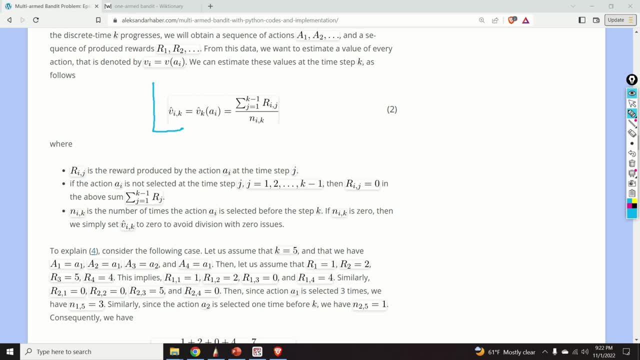 and the index, i is the action number and k is the time step. So what do I do over here? I basically take rij and this is basically the reward produced by the action ai at the time instant j. So what I do over here? 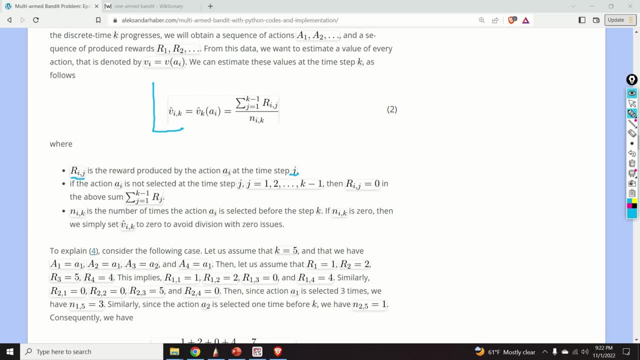 I sum all the rewards produced by certain actions. Now, if the action ai is not selected at the time, step j, then the corresponding value over here is equal to zero, and I will explain this in a sequel Now. n, i, k is the number of times. 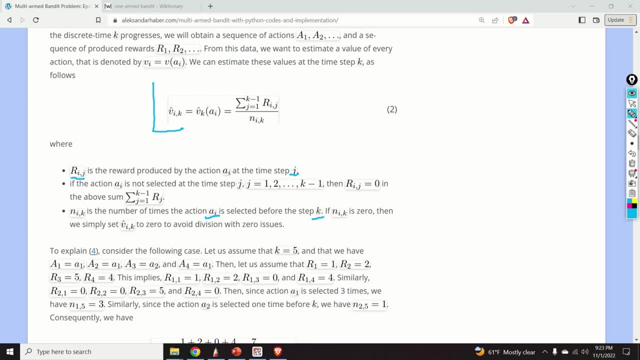 the action ai is selected before the step k. If this value, that is the value of n i k, is zero, then we simply set v i k to zero to avoid division with zero issues. So again, what do we do over here At the time? step k: 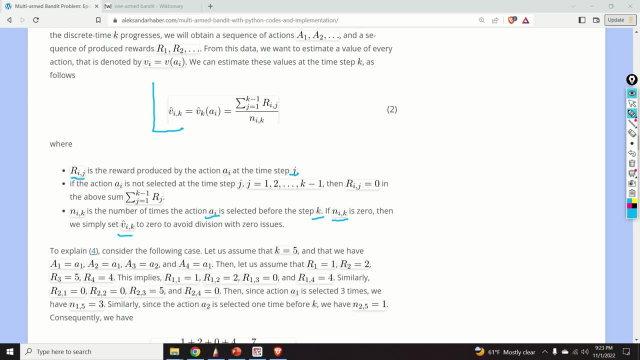 we take all the actions produced by the, actually all the rewards produced by the action i, we sum them and we divide them by the number of times the particular action ai is selected in the time interval from one, two, three until k minus one. To better explain, 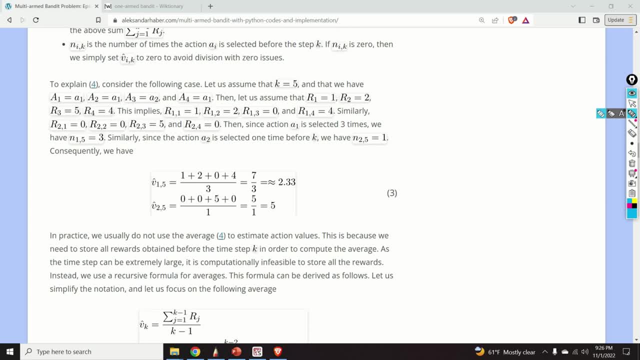 the formula. let us consider the following example. Let us assume that the time instant is, k is equal to five, and let us assume that we have two actions. We have action a1 and the action a2.. Then let us assume that at the time steps, 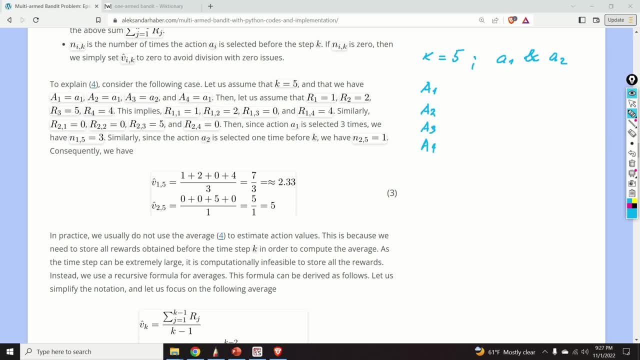 one, two, three, four. the actions were a1, a1, a2 and a1. And these actions produce the rewards, the numerical value values of rewards that are given over here. So they are one, two, five and four. Now this implies that r1. 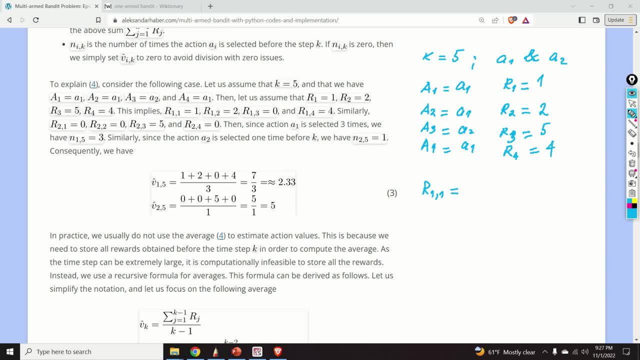 one is equal to one. So at the time step one, the reward produced by the action, one is equal to one. Then we have that r1, two is equal to two. Over here that at the time instant two, we selected the action. 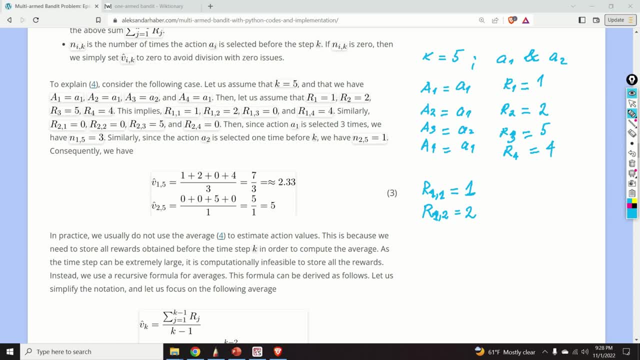 one and here is the index one, and basically the reward is basically equal to two. Then what do we have at the time step three for the action one, for the reward produced by the action one, we can see that at the time instant three, we selected 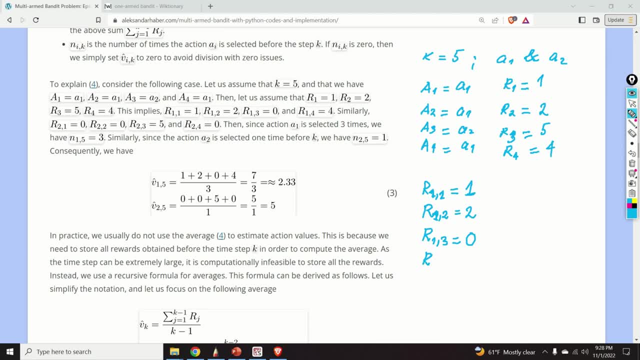 a2.. Consequently, the reward. what do we have for r1, four, That is, what is the reward produced by action one at the time step four? We can see that, indeed, at the time step four, we selected a1 and we obtained four. 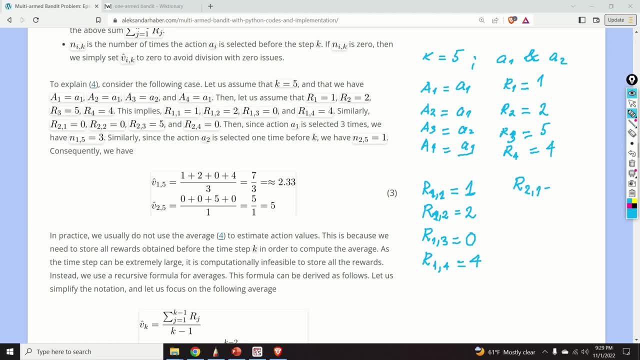 Now, how about the second action? What is r2 one? So at the time step one, we selected action one here. How about r2 two? Again, at time step two, we did not select action two, so we will have zero over here. 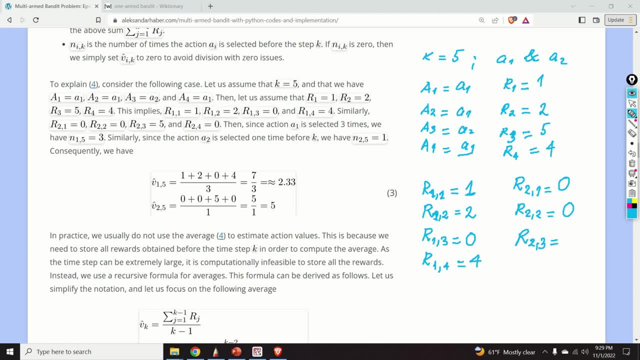 However, at the time instant three, we have actually selected the action number two, so we have five over here. and at the time instant four, we didn't select action number one, so we have zero over here. So what is now our value of the action? 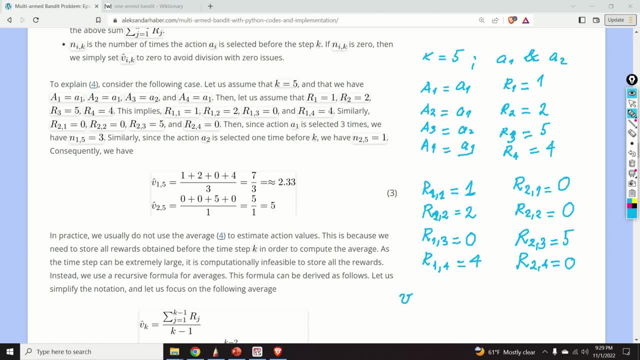 V1, or the estimate. be careful here. this is the estimate of the value of the action One. we can simply obtain something like this: we obtain one plus two or three or three or four, or six, or seven, or eight, or nine or ten or twenty, or. 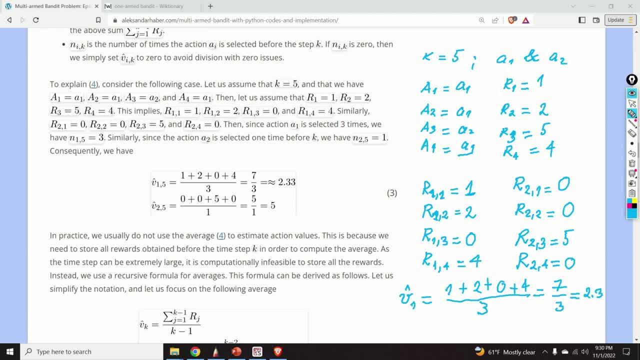 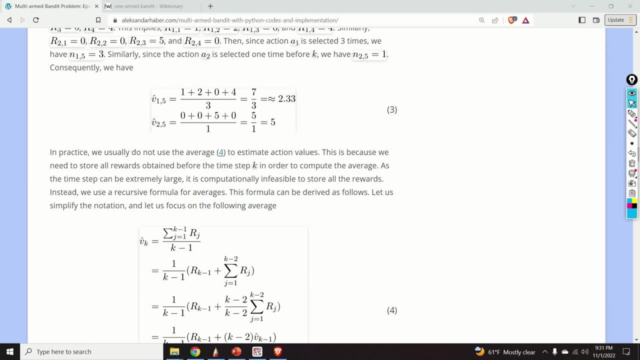 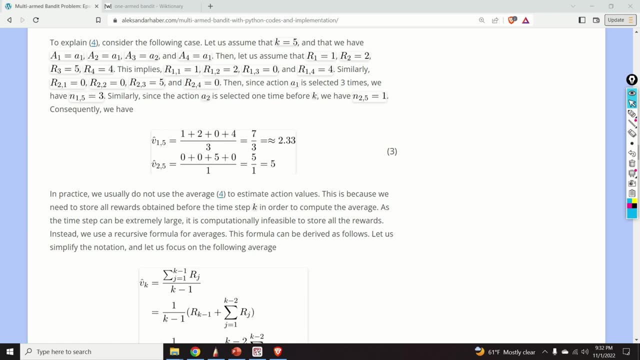 over here. In practice, usually do not use this formula to estimate the action values. This is because we need to store all the rewards obtained before the time step k in order to compute the averages. As the time step progresses, it can become extremely large and it becomes computationally infeasible to 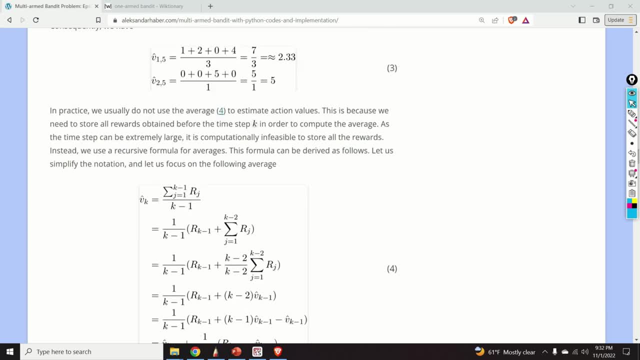 store all the rewards. Instead we use the recursive formula for averages. This formula can be derived as follows: So we can start from our original formula and over here I significantly ease the notation. so just drop the indices of actions. you can later on include them. So what happens over here? 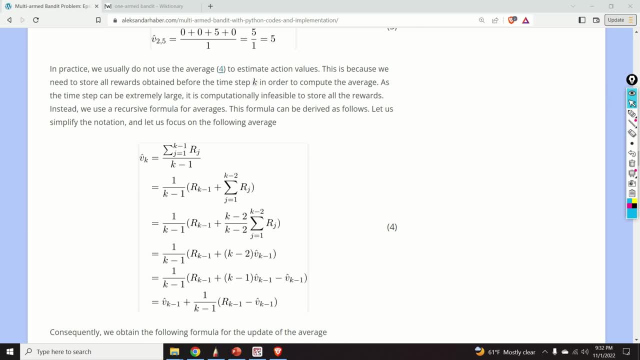 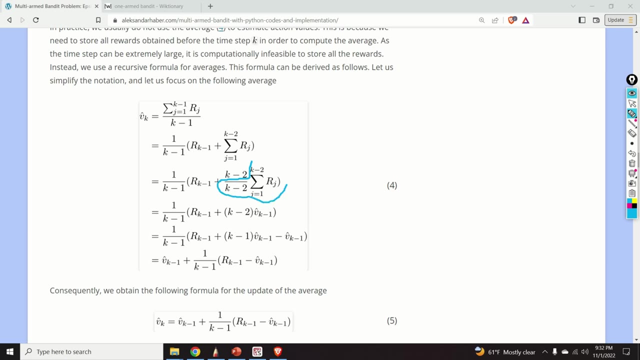 this sum over here can be written like this: basically, if you use the recursive formula to indicate the sum of these has to be, and then you can multiply the term over here by k minus 2 over k minus 2, and here you can observe that the part over here is nothing less than an estimate of. 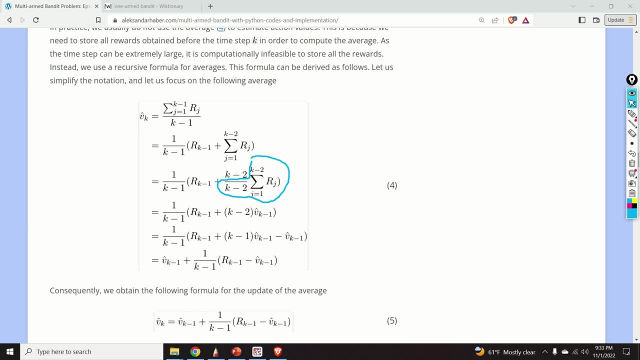 the action, actually the estimate of the value of the action at a time, step k minus 1. and if you kind of split this part over here, you take one of the minuses over here, you put it over here and you kind of massage this equation a. 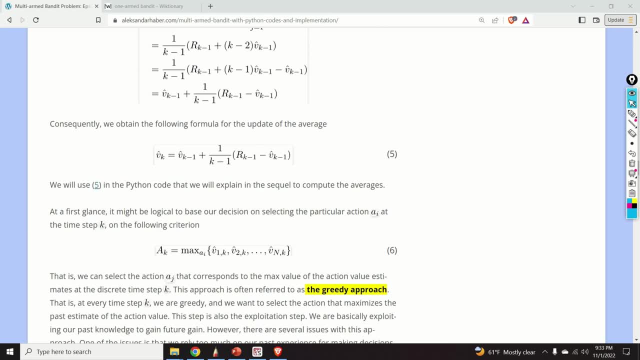 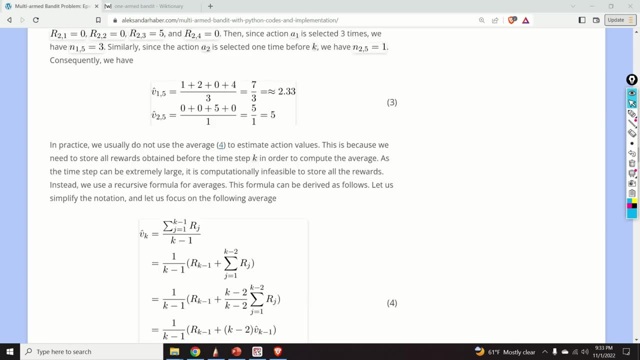 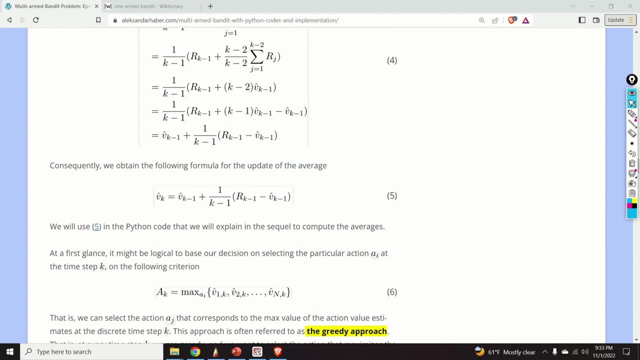 little bit you will obtain this formula or the formula given by the equation number five. so what is the obvious advantage of this formula given by equation number five or the formula given by the equation number two? so obviously over here we only need to remember rise, the previous estimate of the action value. it's basically k minus 1. so 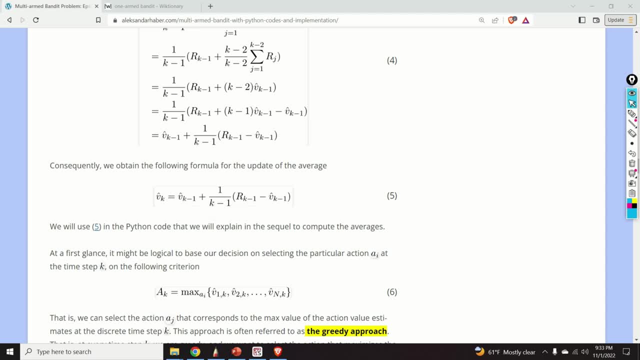 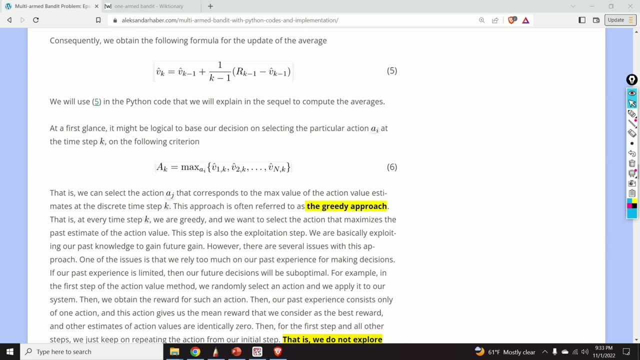 we only memorize the estimate of k minus 1 and we take the reward at the time instant k minus 1, we subtract these two values and we obtain the estimate basically for the time step k, and we will use this formula in the Python code that I will explain. 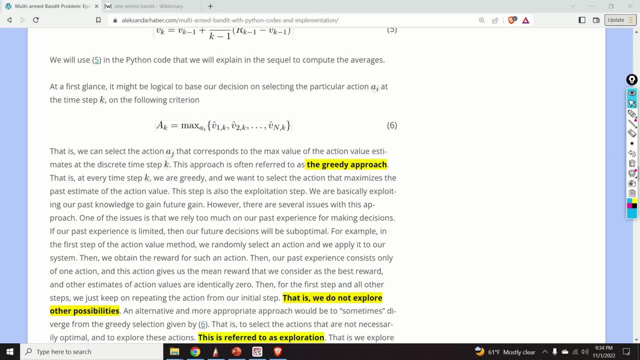 the sequel now. at a first glance, it might be logical to base our decision on selecting the particular action AI at a time- step k- on the basis of the following criterion. so what do we do? we have estimates of the action values right at a time- step k: again we have the estimates of the action value values at: 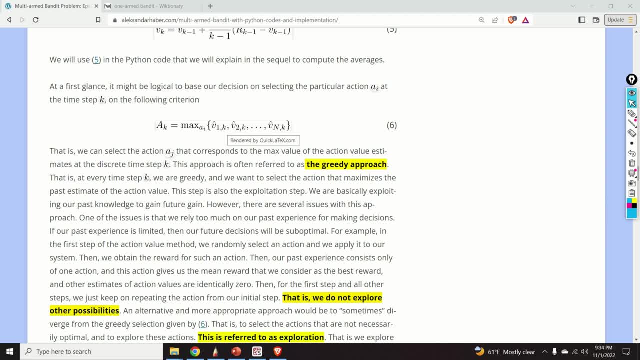 a time step k and but it is the best action. the past action is the action that produces the highest estimate in the past. so we are looking in the past and verde selecting the action that has the largest estimate right, and this approach is often referred to as greeting. 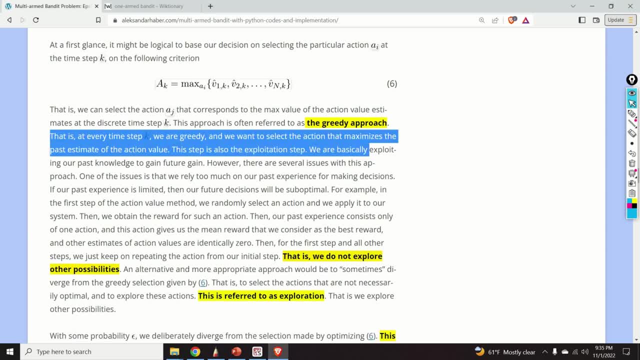 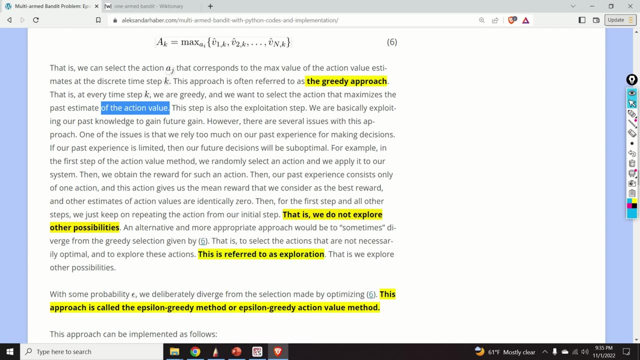 approach. again, i'll repeat this because this is very important and every time step k, we are greedy and we want to select the action that maximizes the past estimate of the action value. This step is also the exploitation step: exploiting something right, We are. 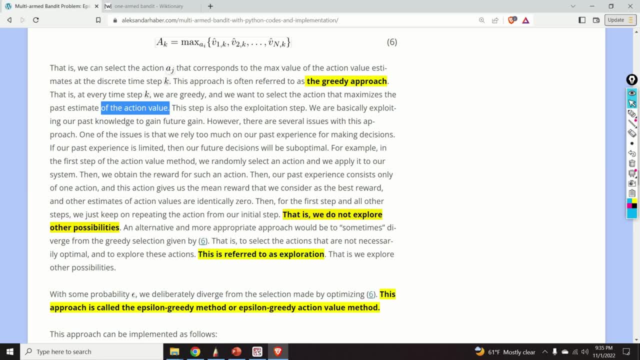 exploiting some knowledge in the past, So we are basically exploiting our past knowledge to gain future gain. However, there are several issues with this approach. One of the issues is that we rely too much on our past experience for making decisions. If our past experience 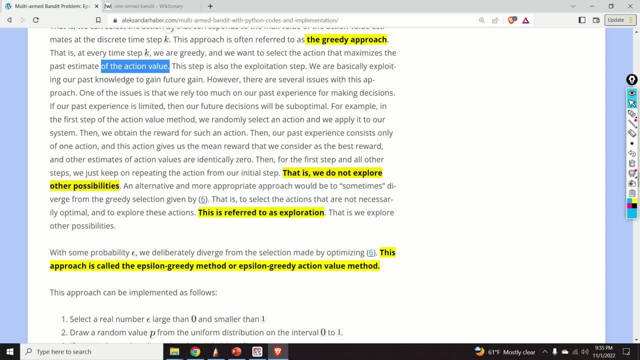 is limited, then our future decisions will be suboptimal. You can, for example, think about the situation In the first step of the action value method. we randomly select an action and we apply it to our system. Then we obtain the reward for such an action. Then 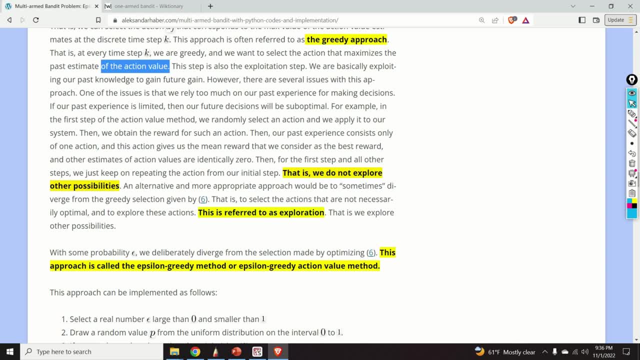 our past experience will be suboptimal, So we are exploiting some knowledge in the past, experience resulting in just one reward: We are basically exploiting some knowledge in the past. Now this action gives us the main reward that we consider as the best reward. 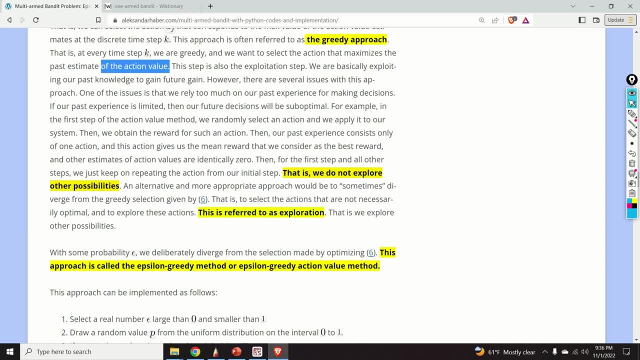 Other estimates of this action value are also zero, Then for the first step, as well as all other steps, we will just keep on repeating the action from our before step, That is, we do not explore other possibilities. This is very important: An alternative and more. 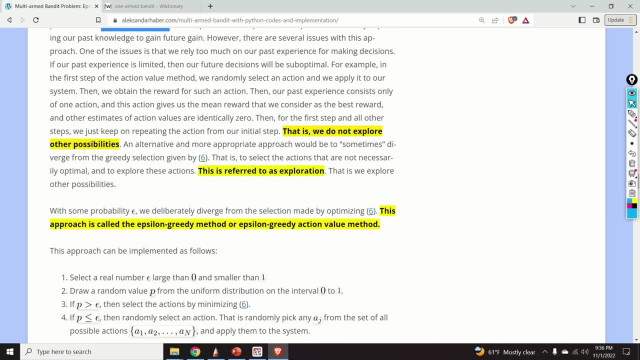 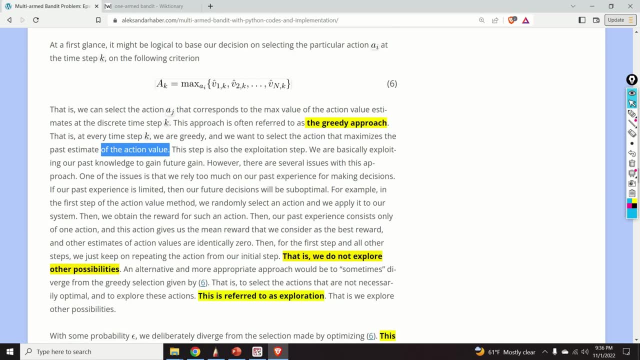 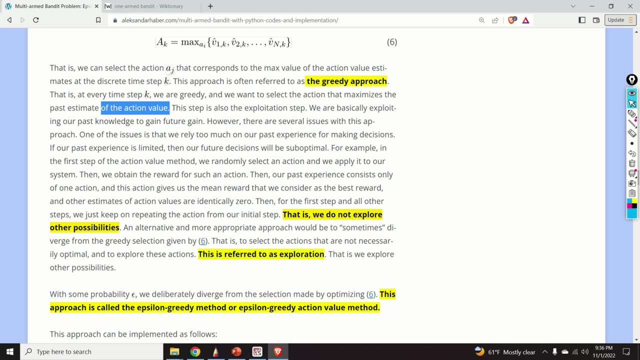 approach would be to sometimes watch out here, sometimes diverge from the greedy selection given by this equation number six, that is, to select the actions that are not necessarily optimal and to explore these under quotes: suboptimal actions. however, this exploration approach might be rewarding, why it will become clear from the future, right, because currently, 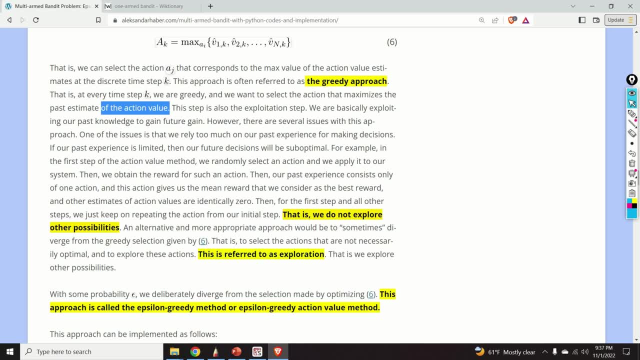 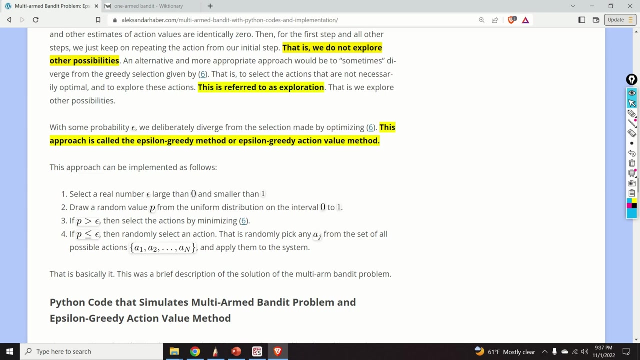 we think that by just minimizing, or actually maximizing, or selecting the actions that maximize the past values of our actions, we are doing an appropriate job. however, this might not be the case, so we want to explore more other possibilities. so what do we do with some relatively small probability? epsilon. 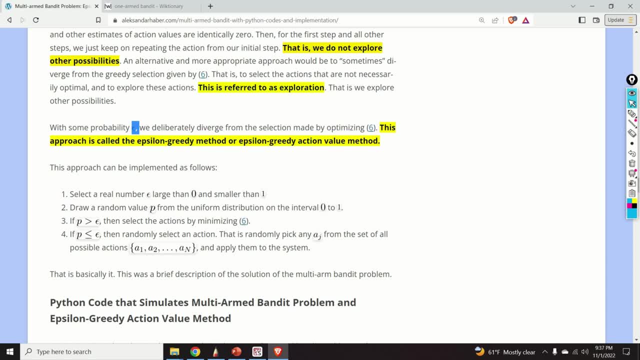 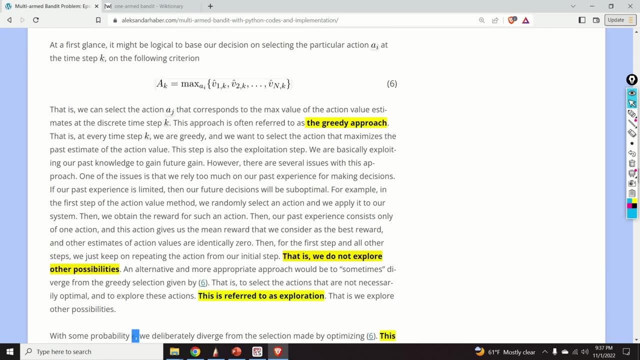 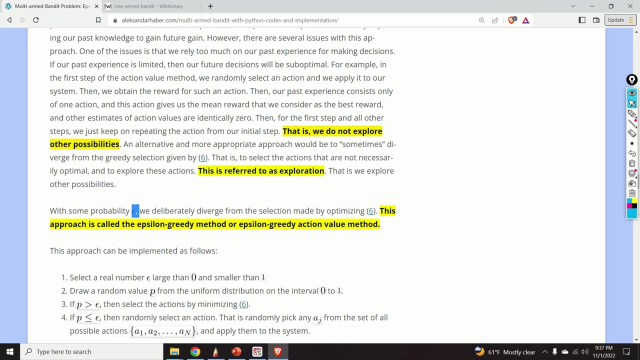 and that's why this whole approach is called epsilon- greedy action value method. we deliberately diverge from the selection made by optimizing six. so we say okay in most of the cases, i will select a k on the basis of this approach. however, sometimes, sometimes, i will diverge, and i will diverge with some probability. epsilon- 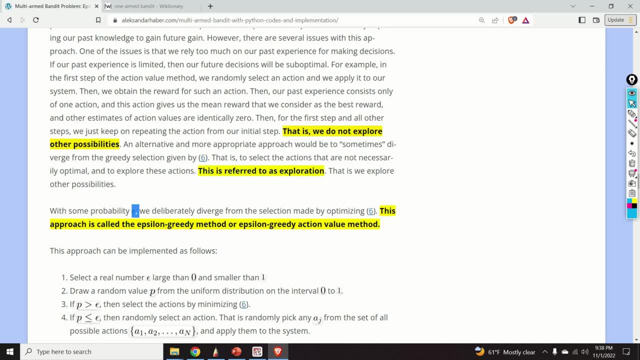 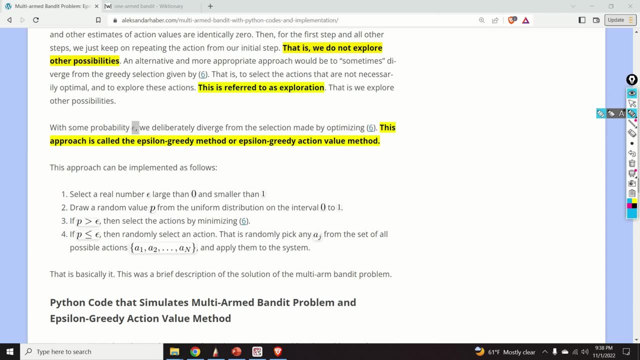 this probability can be zero point one or zero point two. so this approach can be implemented as follows. so what do we do? we select a real number, epsilon larger than zero and smaller than one. so let's say we select epsilon zero point one. then what do we do? we draw a random value, p, and 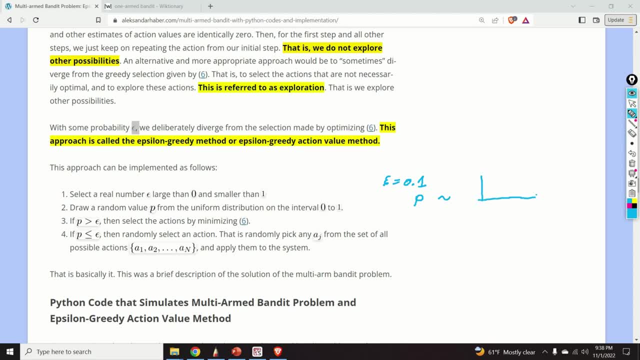 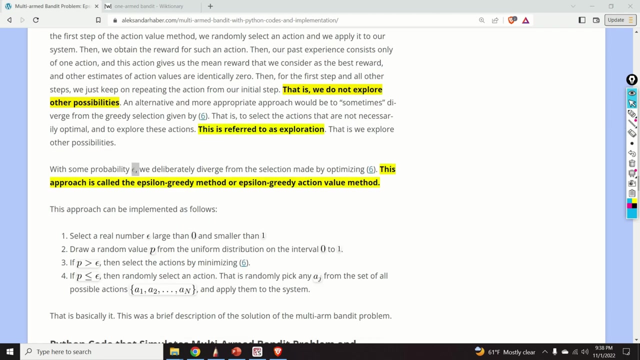 from some uniform distribution, 0 to 1. Now, if this value of P, a random variable, is larger than Epsilon, We basically minimize the criterion 6. so what do we do? we go back and we actually Maximize. I said minimize, I have to correct this in a post. we maximize. 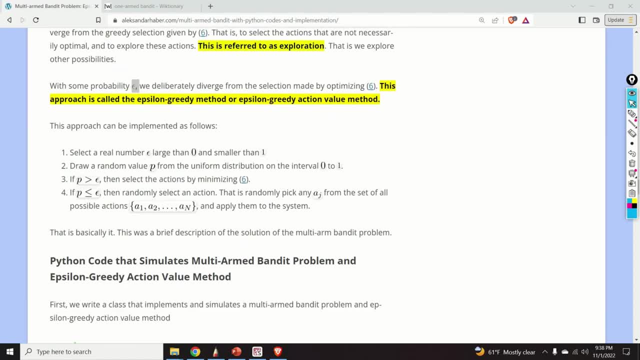 this Criterion. okay now, if probability is smaller than Epsilon, then You randomly select an action. so what do we do if P is smaller than Epsilon? We simply randomly select any action from this set. B, for example, can select a tree, and then we apply this to the system and 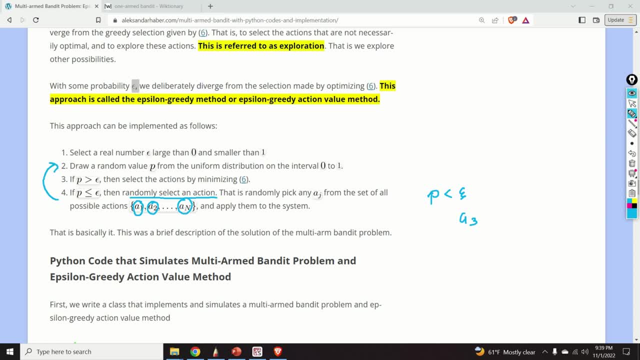 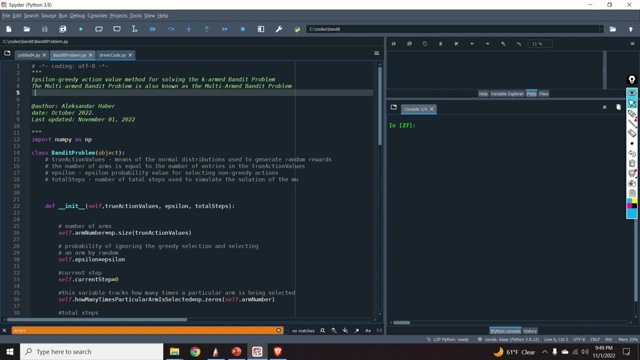 then again we go to the step number, true to. we actually again draw random value P from the uniform distribution and repeat this procedure. In the sequel I will explain how to write a python code that implements and solves the multi armed bandit problem by using the Epsilon Grady action value. 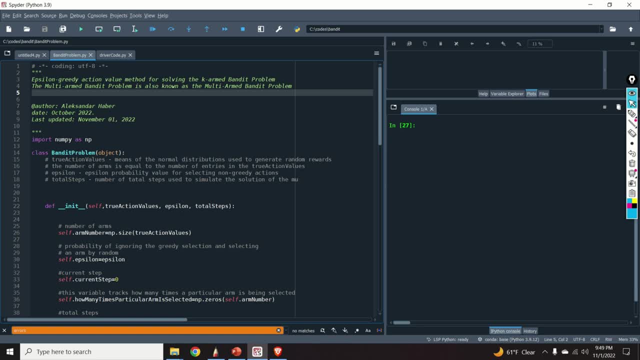 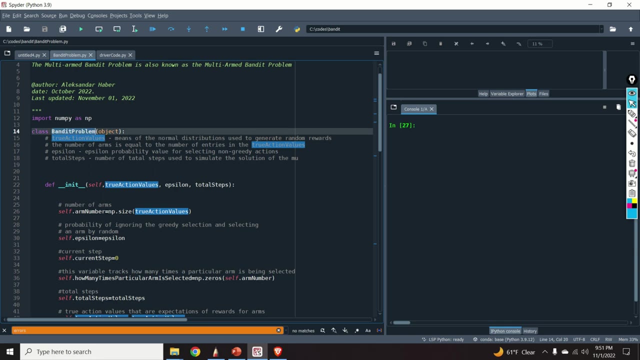 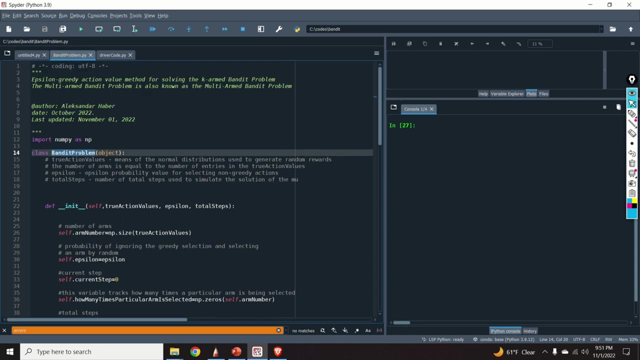 method. Moreover, I will teach you how to write a python code in a disciplined manner, Such that the code can be reusable and easily upgraded at a later stage. The basic idea is to write a class, in my case called bandit problem, That will implement and solve the multi armed bandit problem by using the Epsilon Grady action value methods. 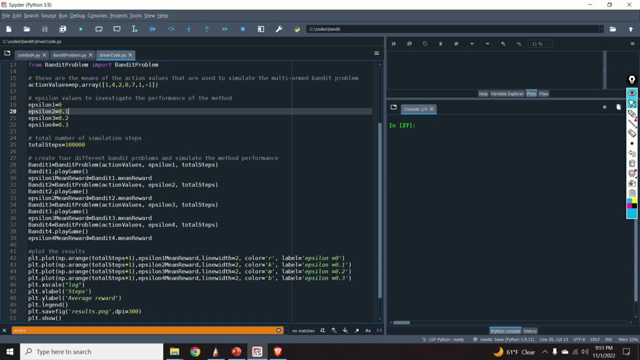 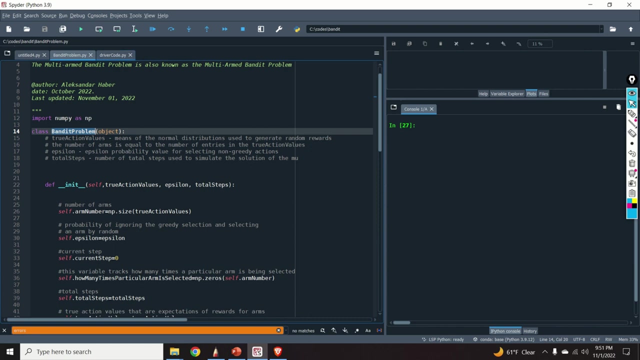 Why I'm writing a class? because In some other parts of your code you can simply initialize and solve the multi armed bandit problem by simply executing these two code lines. So the code is very compressed, It's very easy to read and the class implementation is separated. 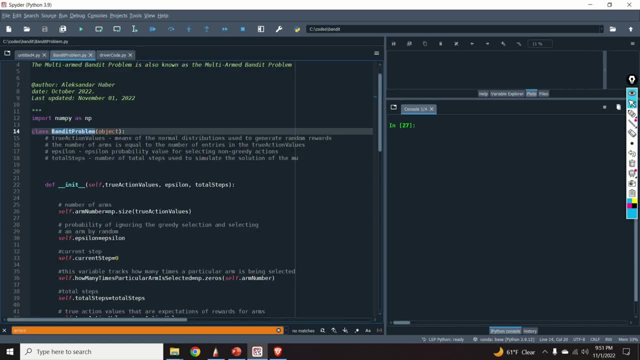 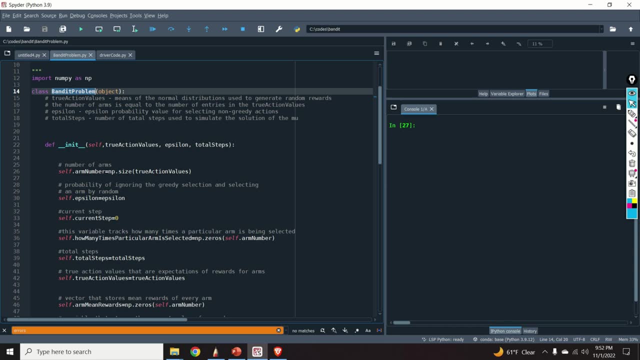 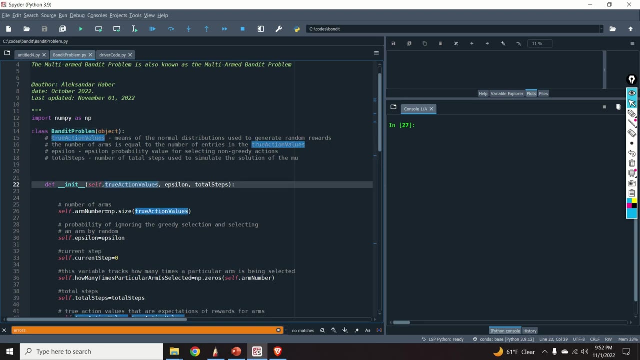 from the driver or from the main code. So let us analyze the variables that we need to provide this to this class in order to initialize the problem. We obviously need to provide the true action values. So again, what are the true action values? The true action values are actually the means of the distributions. 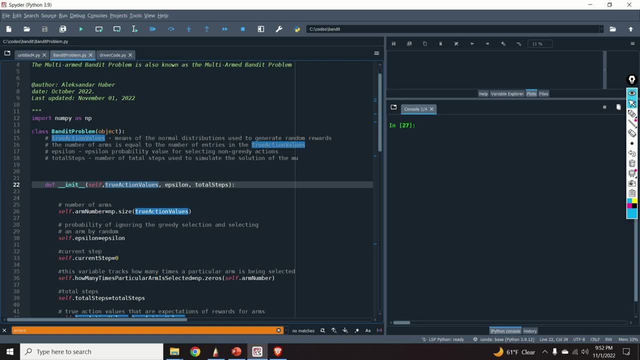 that are created by particular Actions. so, for example, if I select action one, I need to sample my rewards from a certain distribution, and the mean of this distribution is actually an Entry of the true action value. so better to say it like this is that I Entry of the true action value. 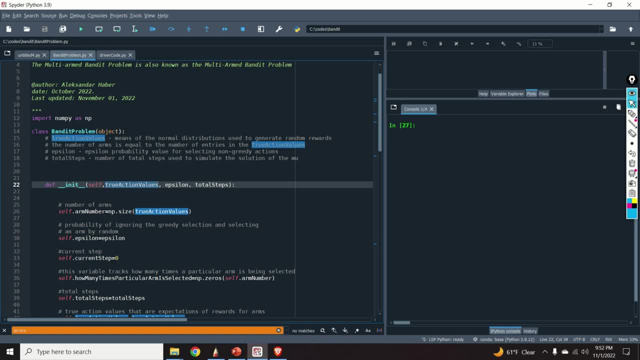 that is the ith entry of this vector over here. that you can see is basically the mean of the distribution corresponding to the action a I. Then the next parameter that we need to provide is To this class is the Epsilon value, and the third parameter is the total number of steps. 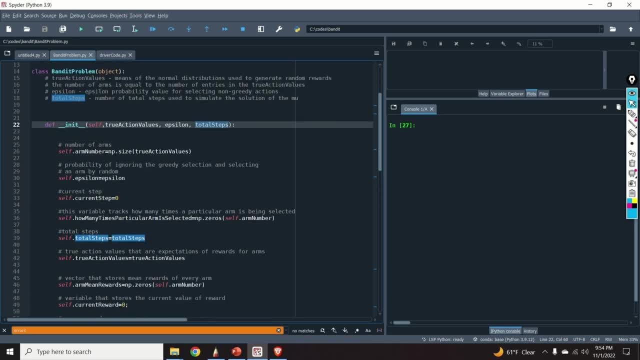 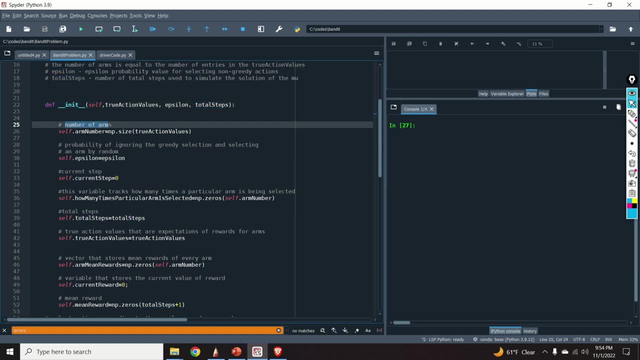 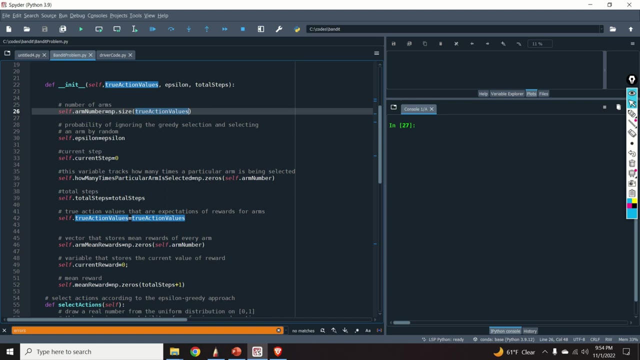 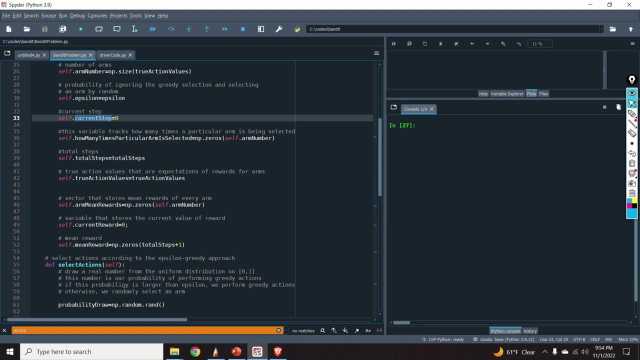 That is the total number of simulation steps. Then in this function, in it we initialize the variables. The number of arms is equal to the size of this vector through action values. Then we basically initialize the Epsilon value, We set the current step to zero And we need to basically initialize another variable, or, better to say, another vector. so this vector. 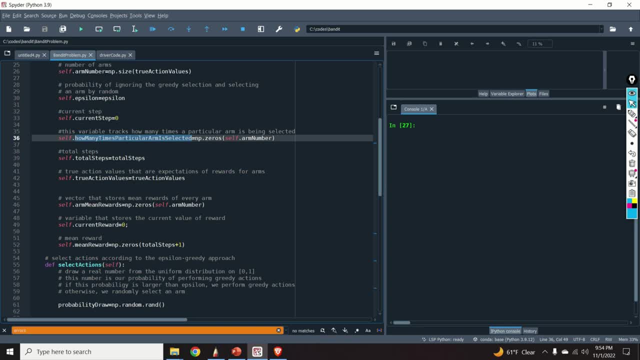 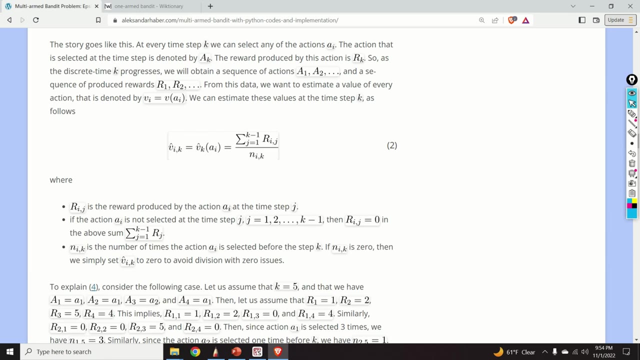 How many times particular arm is selected is initialized as zeros and the ith Entry of this vector is actually equal to this parameter and IK. that is the ith entry of the vector how many times particular arm is selected and Is basically equal to the number of times action I is. 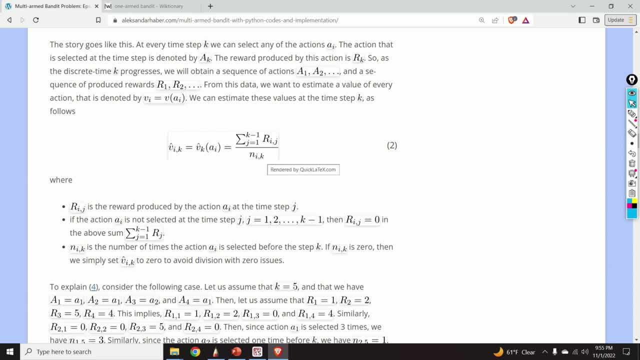 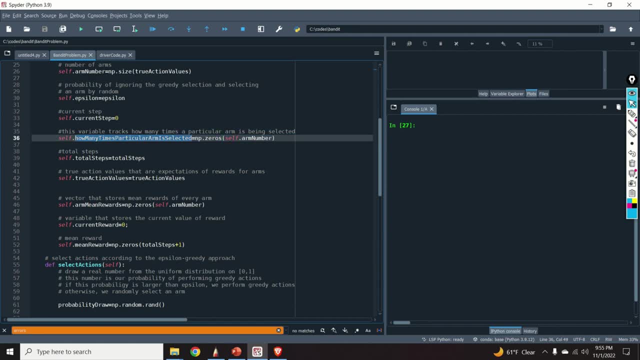 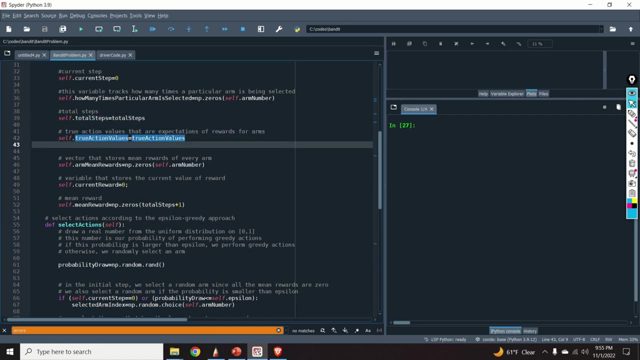 selected prior to the time: instant K. so we need to keep track of NIK and we keep track by defining this vector and by updating the entries of this vector in every iteration. Then we set the total steps And here we basically Initialize the true action values and we simply say: the true action values are equal to the vector. 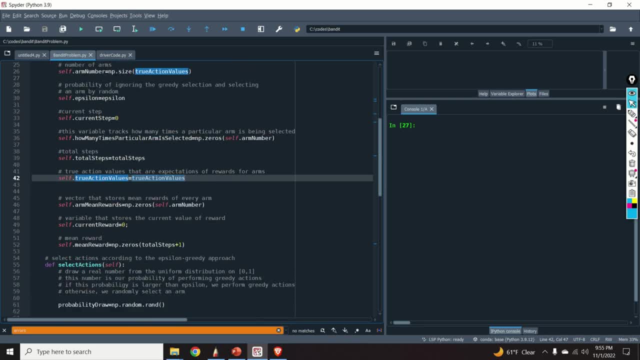 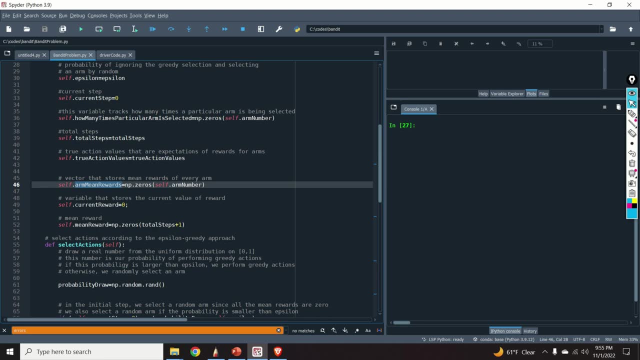 Provided as an input argument over class. Then we need another vector and this vector stores mean rewards for every arm. So if we select particular arm, we will basically obtain some reward by sampling from Distributions whose means are defined in this vector. and when we get this reward, 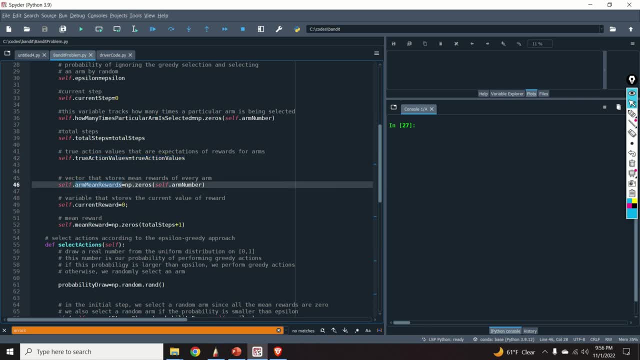 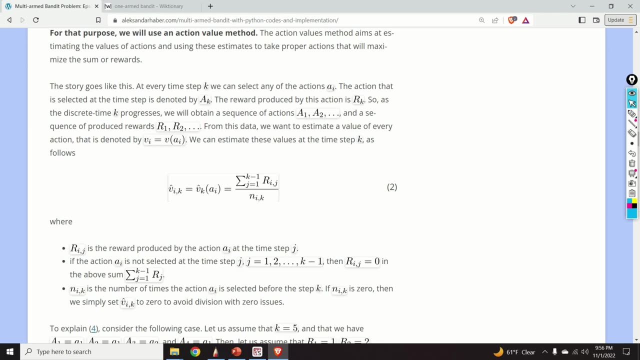 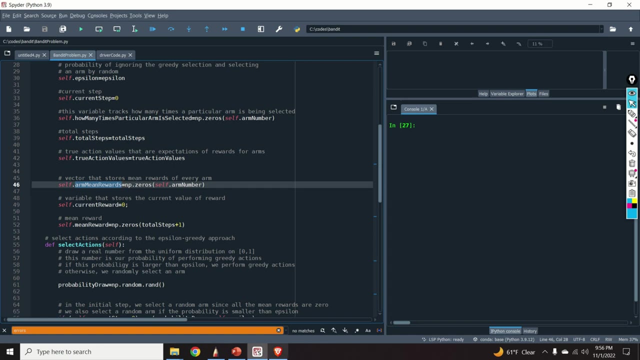 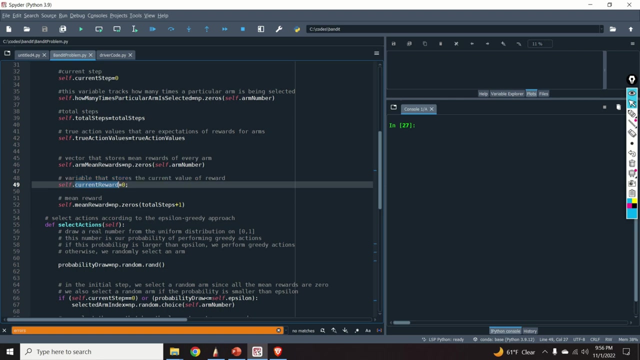 We need to update a mean reward for every arm, that is, we basically need to update the value over here. so the ith entry of This vector- again to repeat, the ith entry of this vector- is equal to this quantity over here. Now we need another variable that stores the current value of reward, and this variable is called current reward and we initialize it by zero. 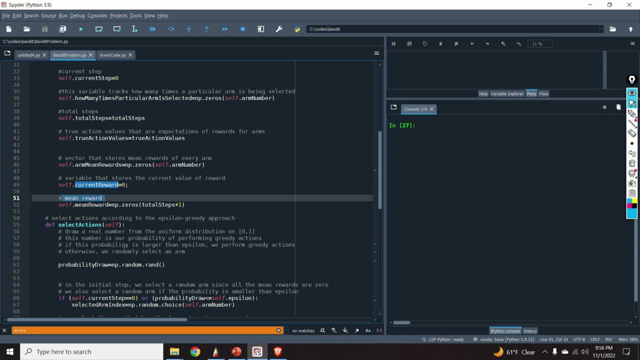 And then we need to keep track of the mean reward of the whole problem and we basically Initialize a vector of zeros where we have total steps plus one Entries and this vector will be populated and later on, when we analyze results, We will look into the entries of the 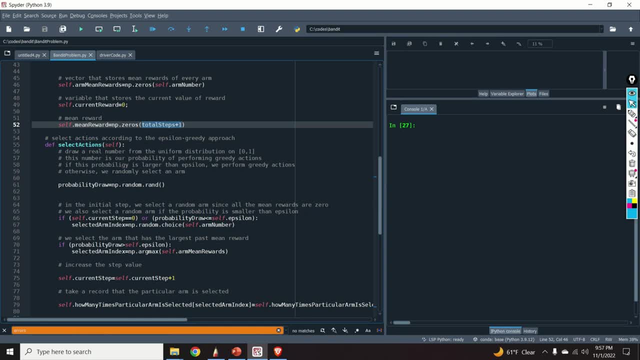 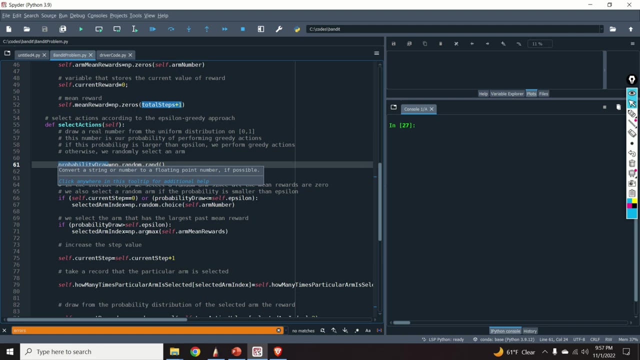 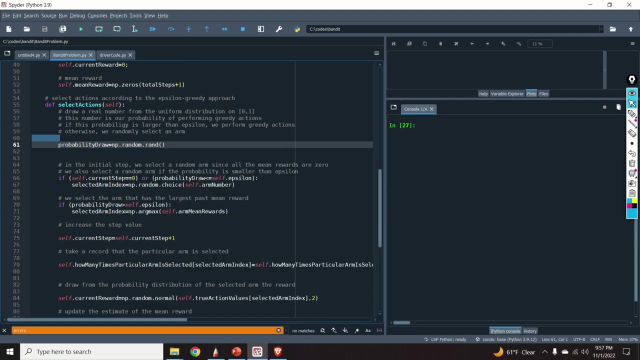 Factor. Next, we define the function called select actions, and this function basically implements an Epsilon greedy approach for solving the problem. So what do we do over here? We basically first randomly select a number from a uniform distribution defined on the interval of 0 to 1. 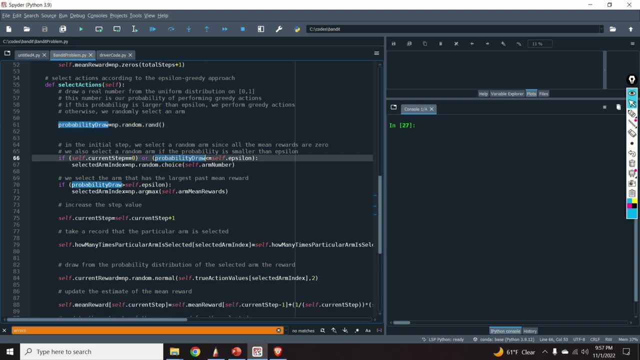 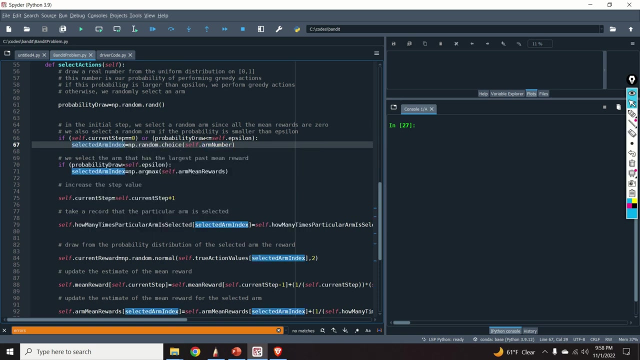 now we analyze this vector. If this value is smaller than Epsilon, then we perform The exploration step, that is, we don't use the greedy method. This means that we simply randomly select the action and This index will correspond to the index of the selected action. on the other hand, if the probability is larger than Epsilon, then we basically perform a 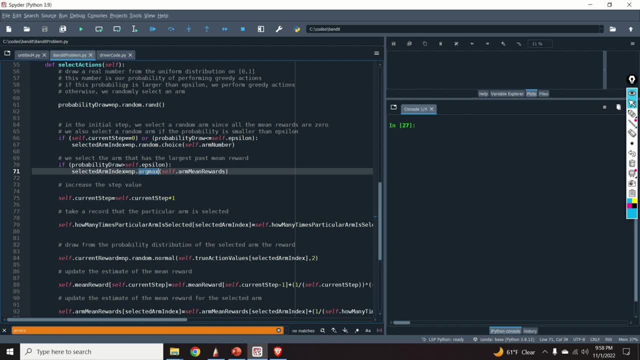 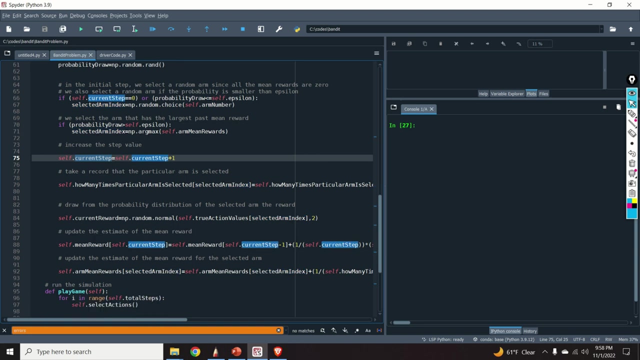 greedy approach. we find the index of basically The our mean rewards, the mean rewards that maximizes an estimate and this is our index corresponding to greedy actions. then we increase the step value and Then we take a record that the particular arm is selected, that is, we simply update. 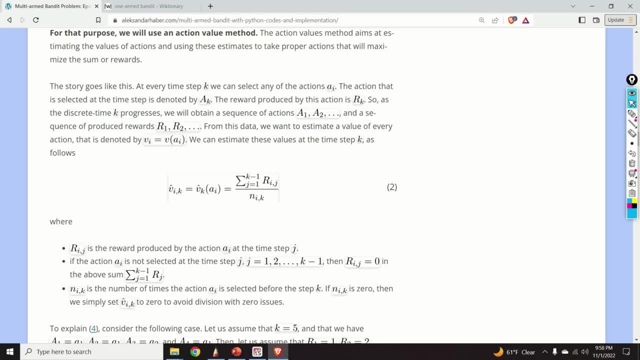 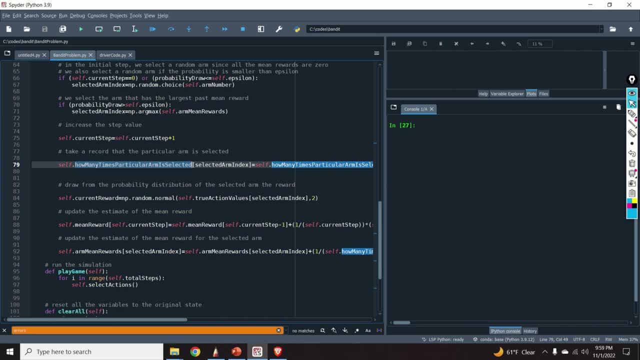 This vector over here actually entries. this is the entry of The vector and we simply update it over here. Next, we draw from the probability distribution of the selected arm to get the reward. So we simply say: we simply draw from a normal distribution where the mean corresponds to the mean of the. 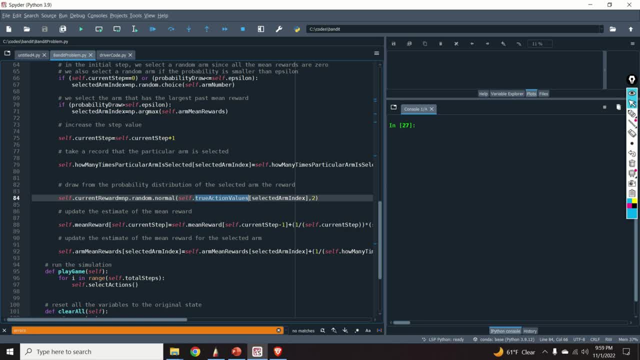 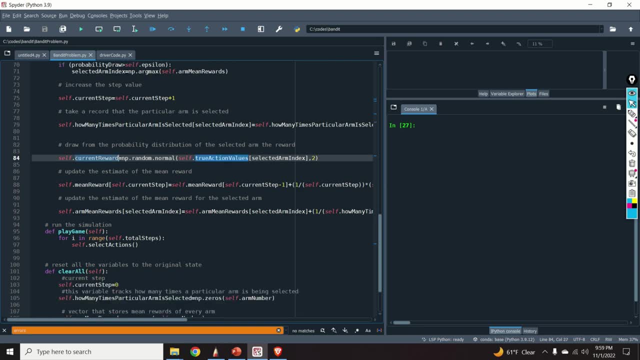 selected, basically action, that is the mean of the probability distribution For the particular or for the selected action. we get the current reward, then we update the estimates of the mean reward and We update the estimate of the mean reward for the selected arm, and that would be it. 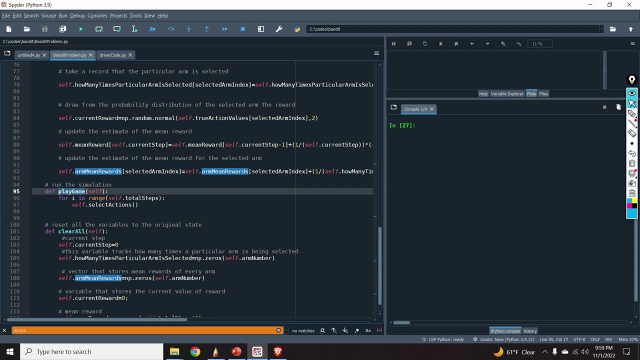 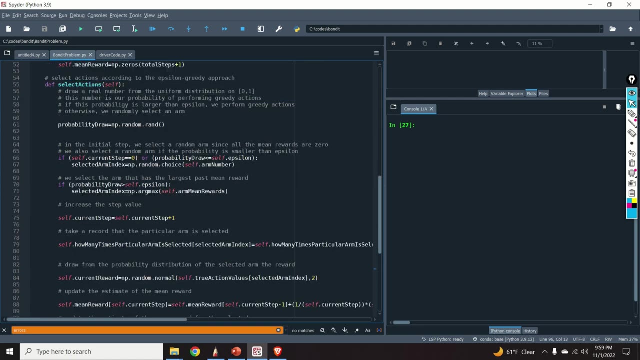 Then we define the function that plays the game. So what do we do? we introduce a variable I that goes from 0 to the total number of steps and We simply, in every step, we select actions. We simply call This function over here that updates the estimates, that selects random values. 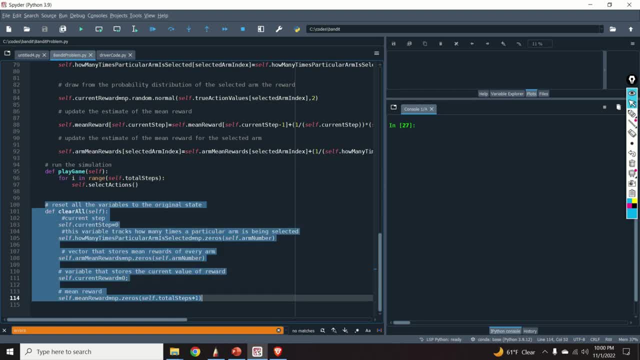 Etc. And Finally, we can write a function that basically resets all the values or sets them to 0. This function can be used if we want to play this game from the beginning, So we need to reinitialize all the values and to set them to 0. 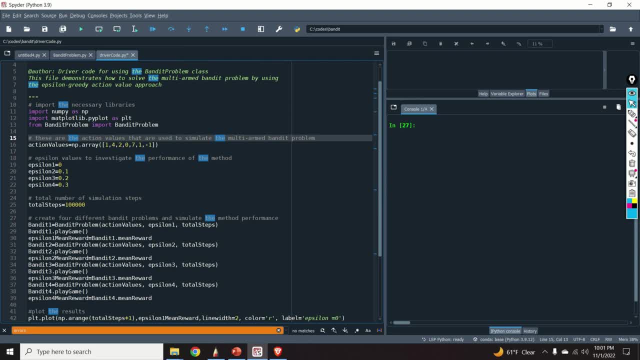 Let us now explain how this class can be used in other codes. The first step is to import the necessary libraries. We import the numpy library, then we import the plotting library, and from bandit problempy, That is, from this file, We import our class, and over here I'll just save. 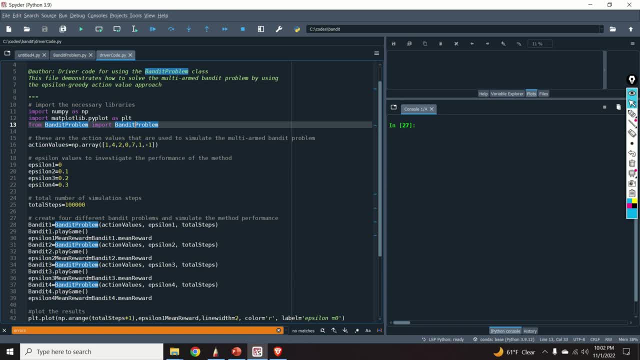 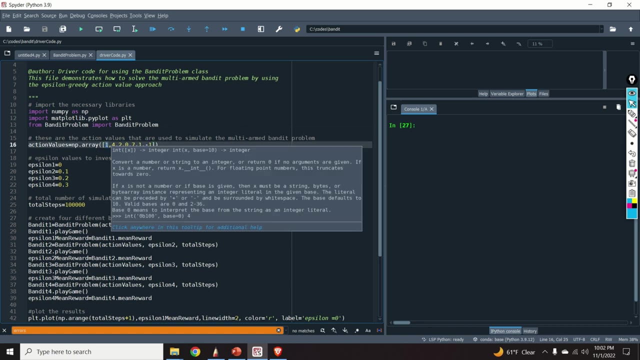 my code to avoid any problems in the future. Now the next step is to select the action values that are used to simulate it, to simulate the multi-armed bandit problem. so we select Action values as 1, 4, 2, 0, 7, 1 minus 1.. We assume that we have 1, 2, 3, 4, 5, 6, 7. 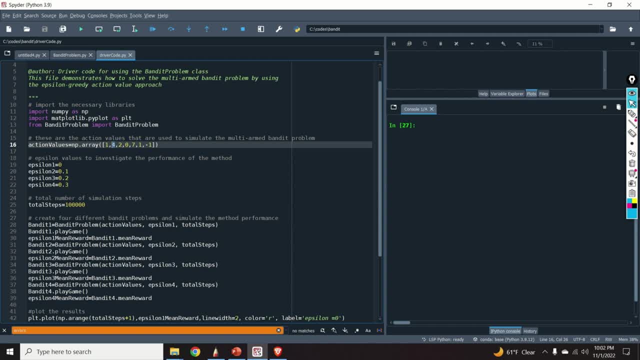 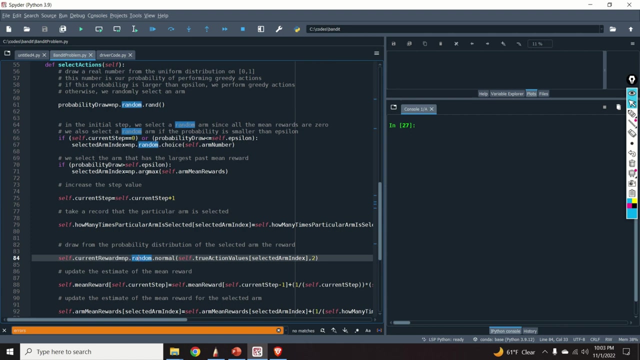 arms, and basically every entry of this vector corresponds to the mean value of The distribution created by certain action. so for example, over here For the action number 3, the mean value of the distribution will be 2, and in our class over here we basically. So let me just for a second locate where we do that. 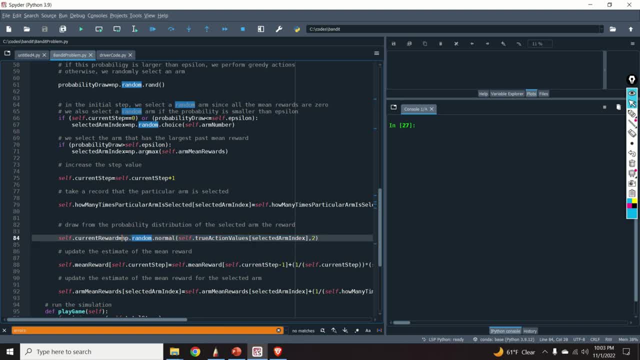 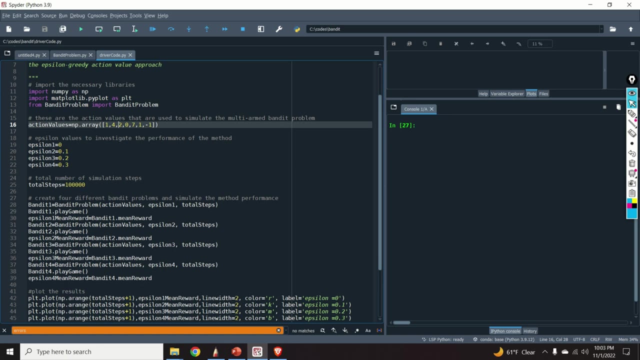 That is, we do it over here. We basically select a random value of reward from a certain distribution whose mean is actually defined over here. The next step is to select Epsilon values. we select different Epsilon values to investigate the performance of the method, and you will see later that the performance of the method 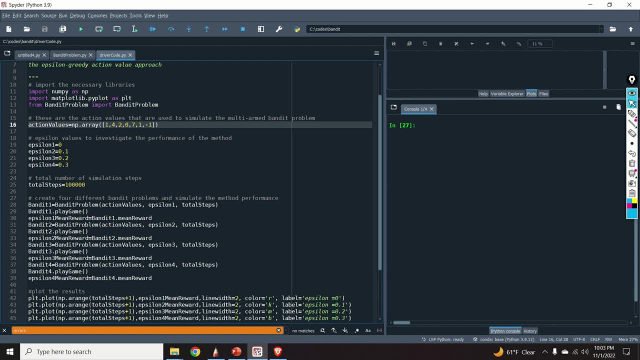 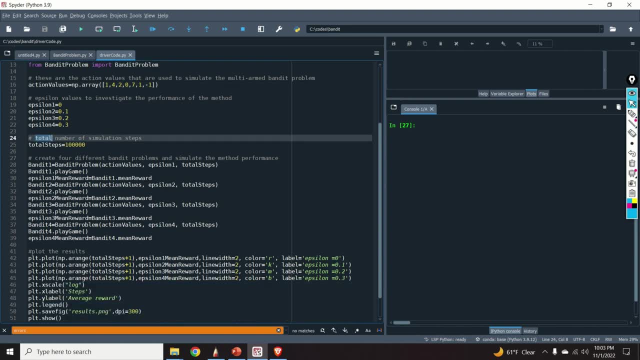 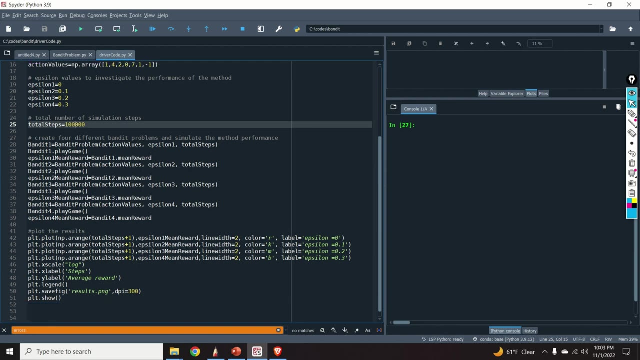 highly depends on the Epsilon value. so we start with zero, we increment the Epsilon values to, with a step of 0.1. Then we simulate the problem for 100,000 steps. Then over here we create four banded problems. Every problem is defined for a certain value of epsilon. 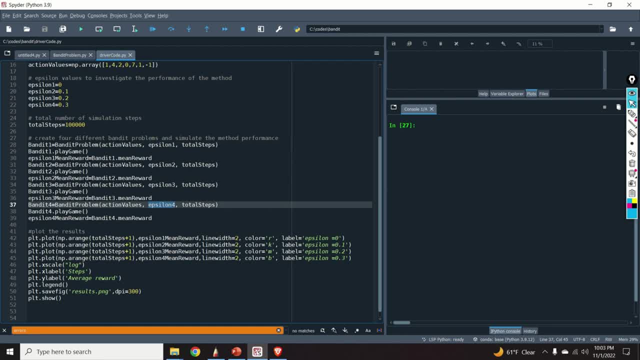 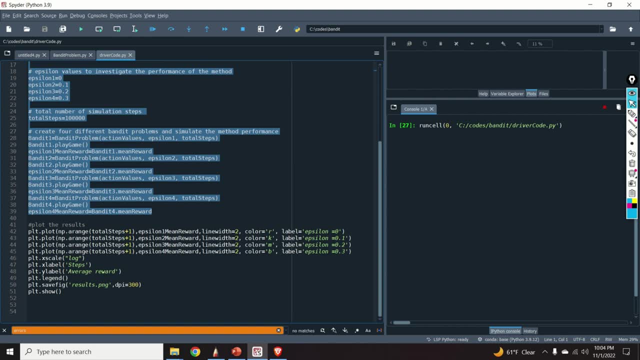 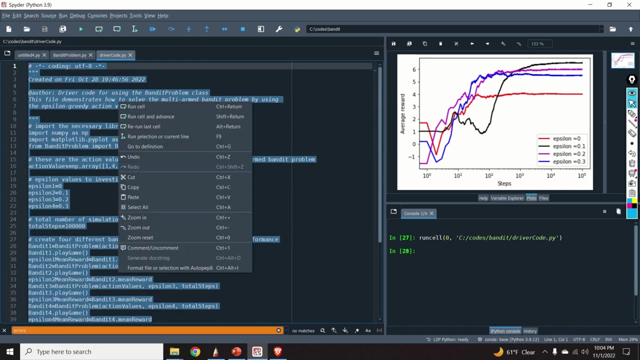 Epsilon 1,, epsilon 2,, epsilon 3, and epsilon 4.. And let us execute the code and let's see what will happen. Okay, now I executed the code and obtained this result over here. Notice that, basically, while doing this, I press the right click and instead, basically, 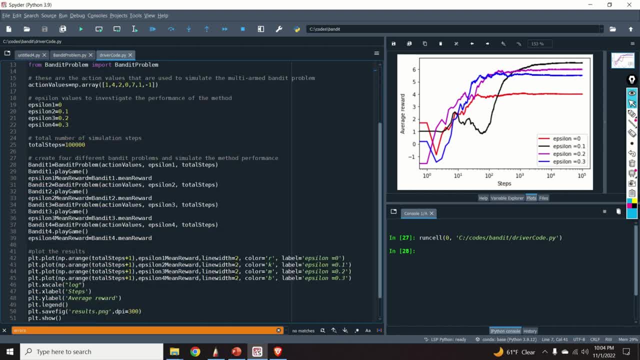 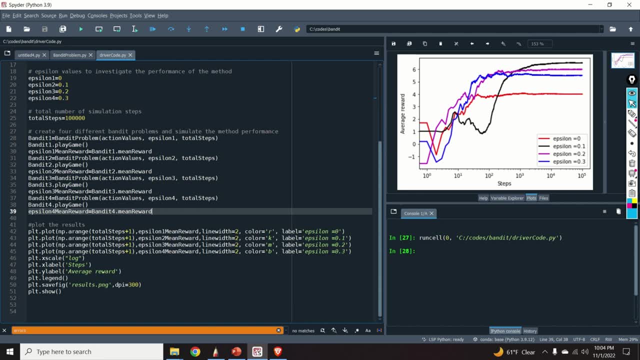 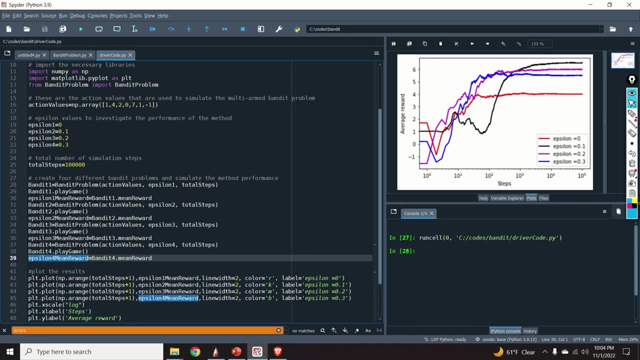 clicking over here. I clicked over here. This means that the code executed from here until here. However, I wanted to do something else. I wanted to execute my code from line 1 until line 39. So I will repeat the step. I will erase my workspace. I will also erase. 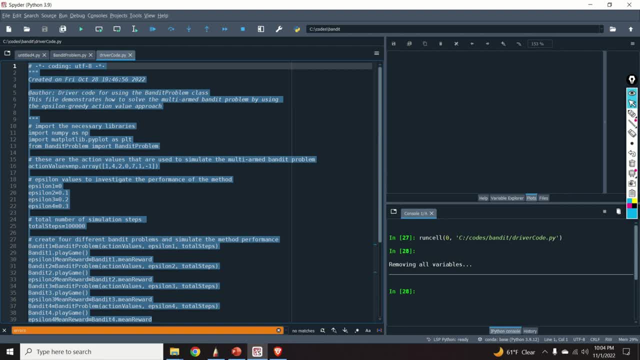 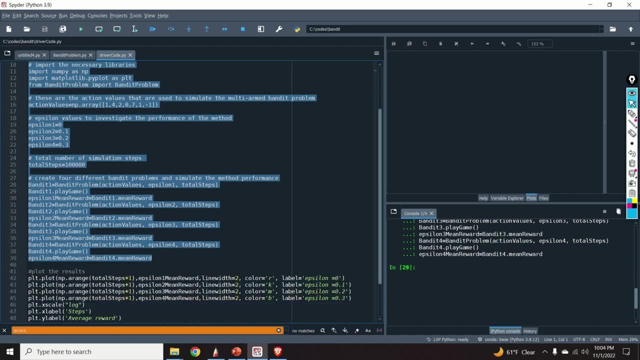 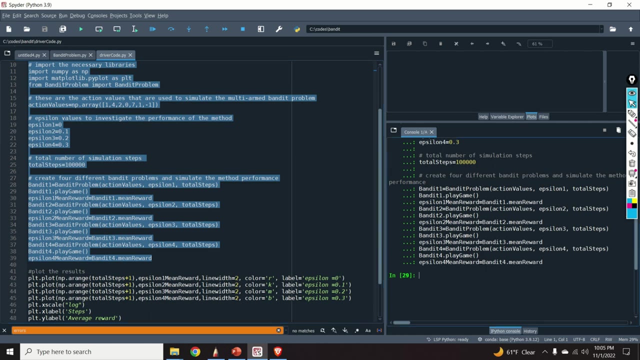 the part over here and then I will perform the correct step. So I will select over here and I will do this. It takes some time. It's quite fast On my computer. I actually have a computer that's one year old, So it's a very good computer. 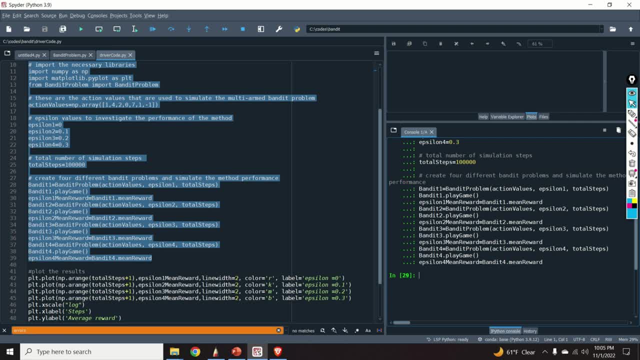 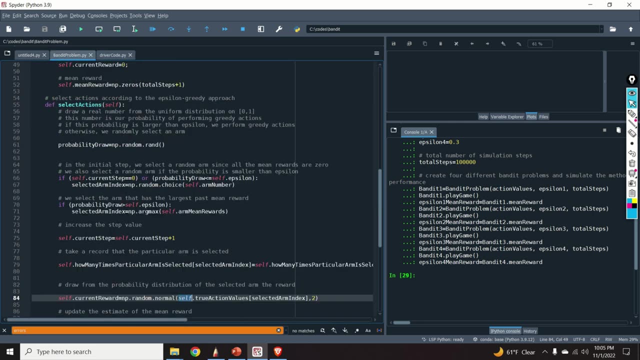 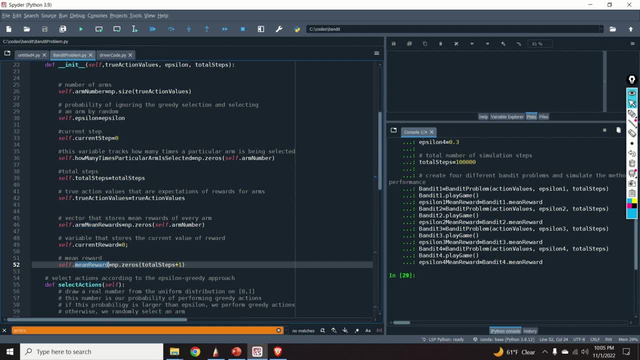 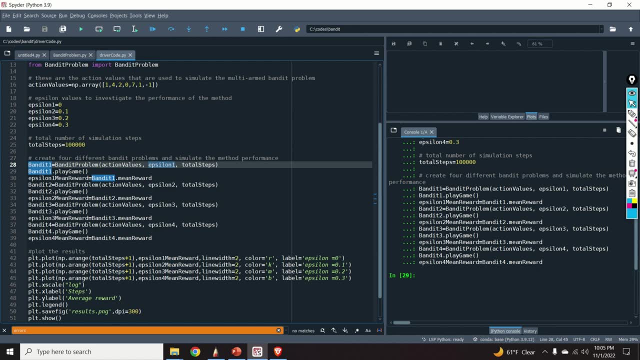 variable that's initialized over here, And another variable is instance none And another variable is the. The mean reward is more important, since it tracks the production of the problem or The solution of the problem for certain value of the epsilon. So what do we need to do? We basically need to plot the. 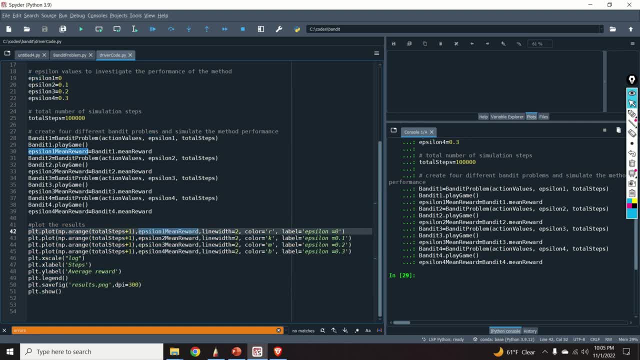 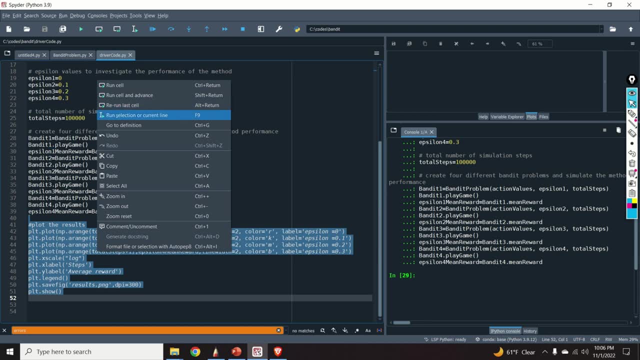 result. So what do we mean? We will basically plot the mean: rewards with respect to time steps for different value of epsilon. So let's see what happens over here. So I would consider that, because this is a very simple metric system and there will be some 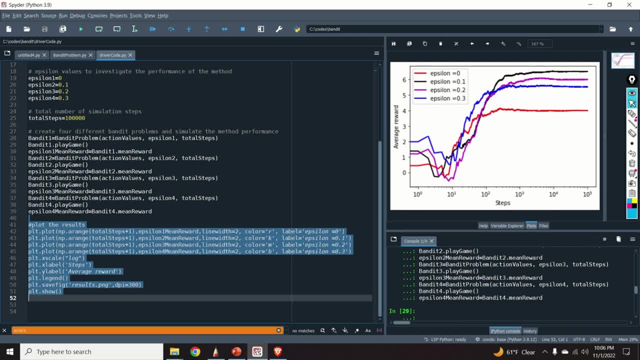 take- longer à la carte onESLierry fringe how it looks. So let's see what happens over here To scheduled driving which will cheering on the left side. and here is the result. here we see, in the logarithmic scale are steps, and over here we see. 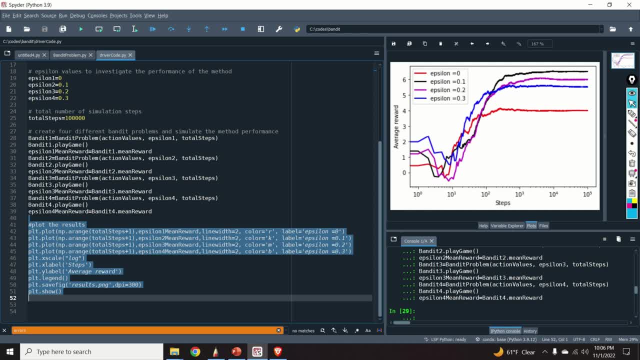 average rewards obtained for different values of epsilon. you can see the red line. that is. the completely greedy approach does not produce good results. it produces diverse results. the best results are produced for. epsilon is equal to zero point one. we can over here see epsilon, zero point one. 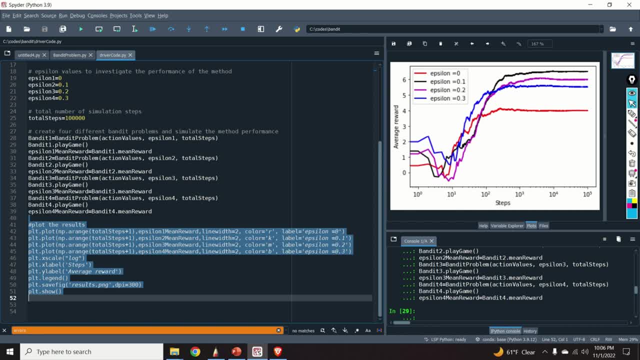 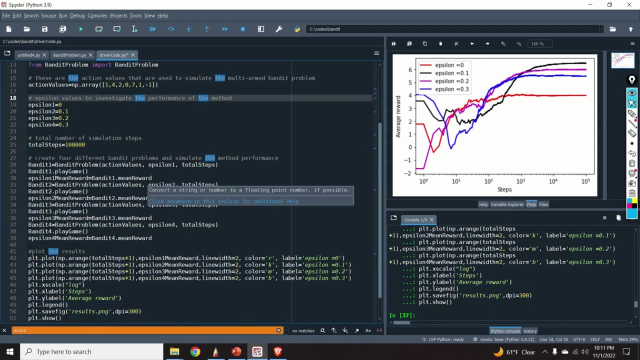 and starts to deteriorate as epsilon increases and we can see for epsilon zero point two, zero point three. we obtain this line over here. let us now briefly analyze the convergence of the solution method, for epsilon is equal to zero point one, that is, we need to extract the mean reward. 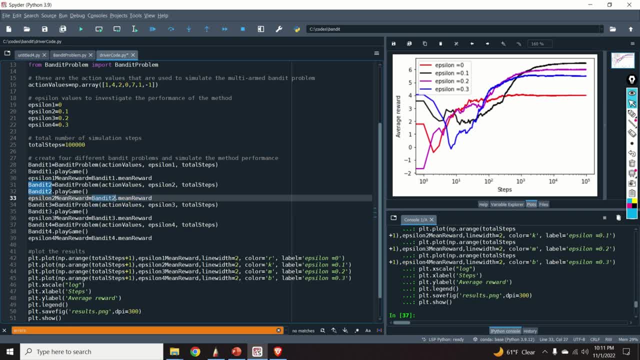 for the second bandit problem. and the mean reward is extracted over here. so let me want aspect or let me just show this factor. in this window we can't see that this factor converges to the value six point for ink. so this is the mean and i'll going back to our action values. 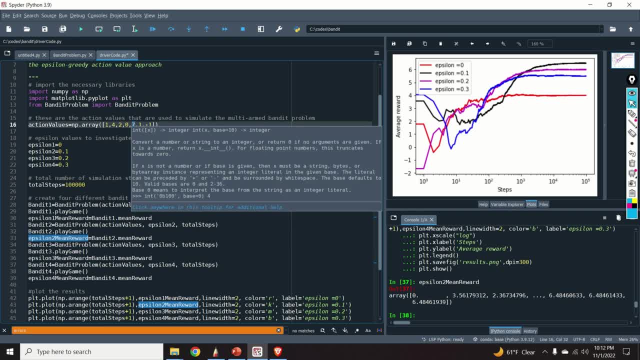 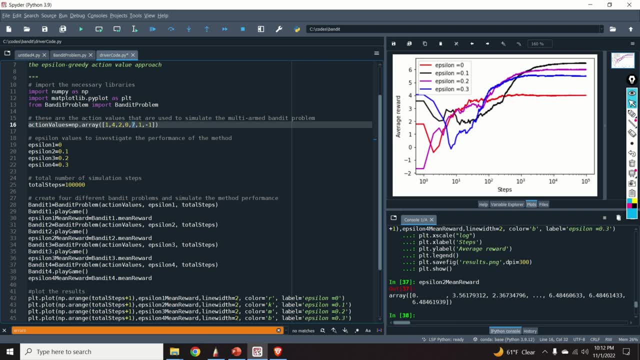 we can't see that this e reward is actually very close set and seven is actually the maximum value of the action value. that is, we can see that our mean reward converges to the action value for the action 1, 2, 3, 4, 5, and this is a good 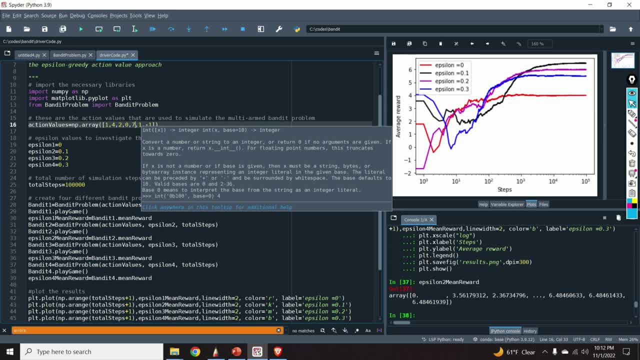 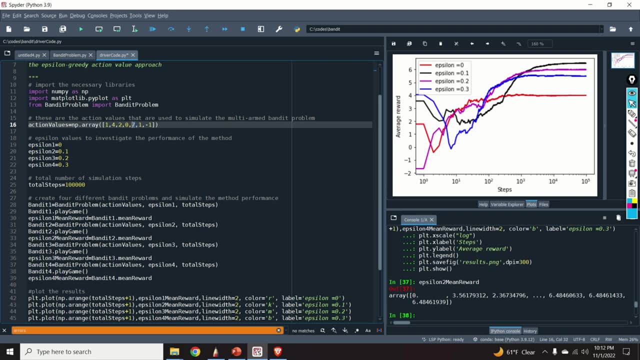 check of the implementation accuracy, because somehow logic tells us that the best option is always to choose the action number 5. why? because the action number 5 will produce the highest action value, and this action value is equal to 7, and we can see that our mean reward is close to that value. now we can do further. 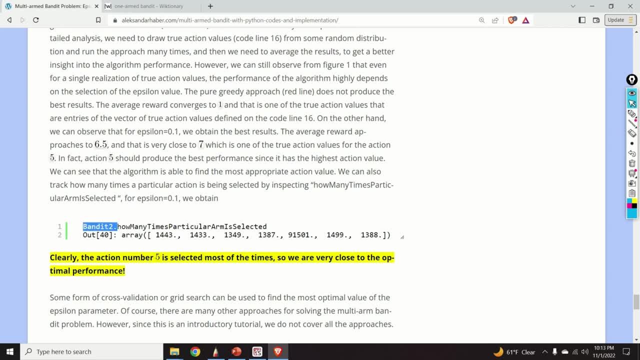 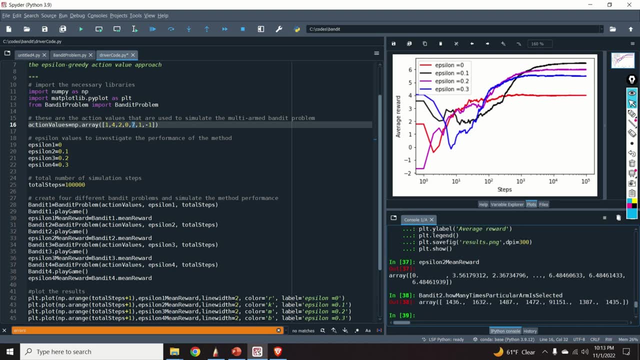 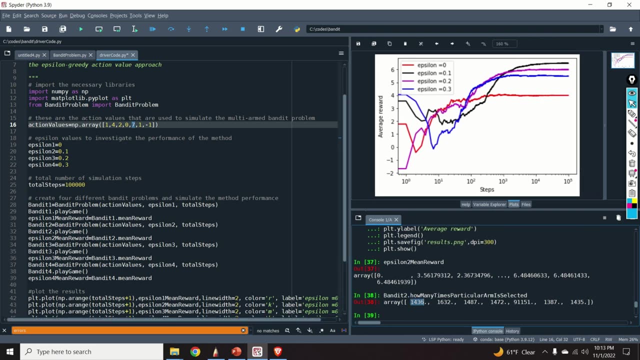 investigation and we can basically try to see how many times particular actions are selected during the simulation process. we can see that the action one is selected- 1436 steps- and you can see the numbers, numbers of numbers, of basically how many times a certain action is being selected during the simulation process. 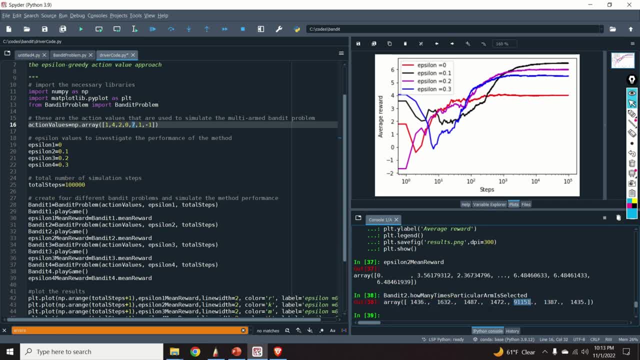 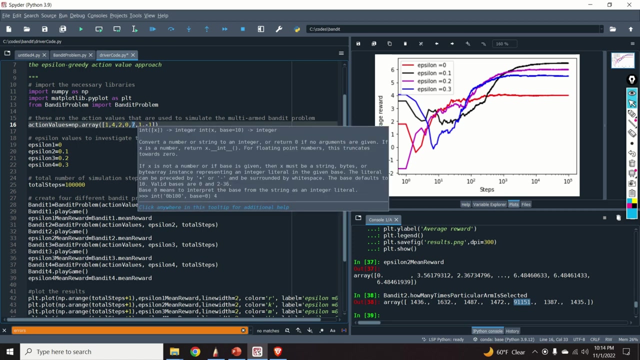 and we can see over here that the action number 5 is selected 91 times 150 you one. so we can see that most of the times this algorithm selected action number five, and action number five corresponds to the largest value of the action value. so our algorithm is doing a good job, for epsilon is equal 0.1, of course, 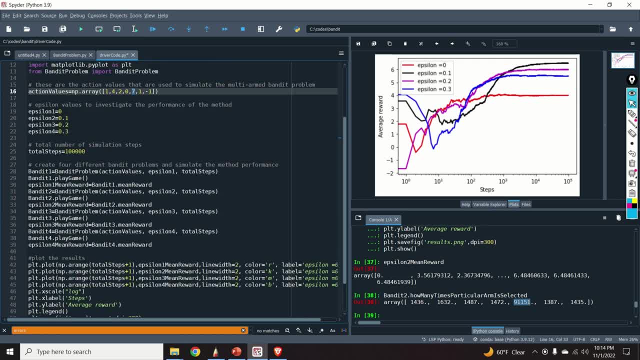 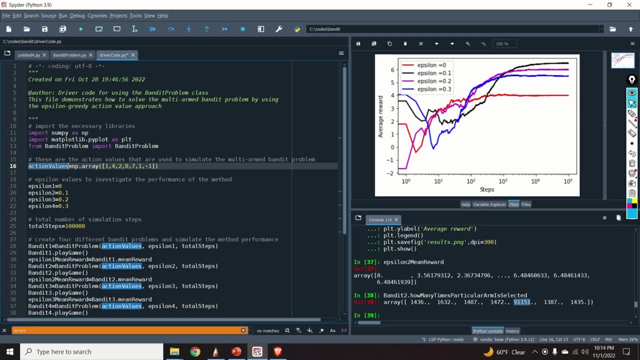 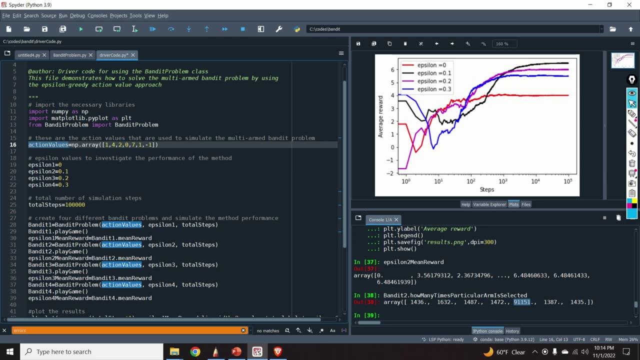 in practice, you would basically need to simulate this algorithm, not for a single realization of action values that I've shown over here, but instead you would need to do that by, for example, writing a for loop, and in every for loop over here you will select certain action values and then, for this action values you will 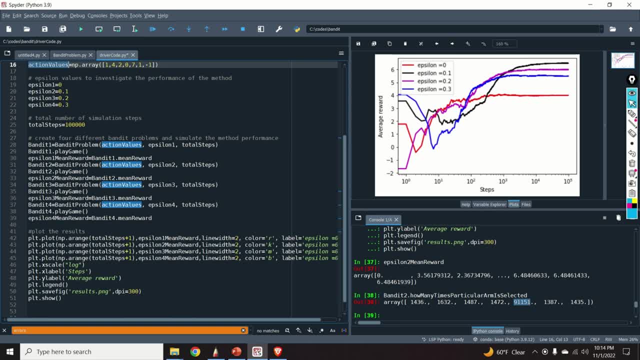 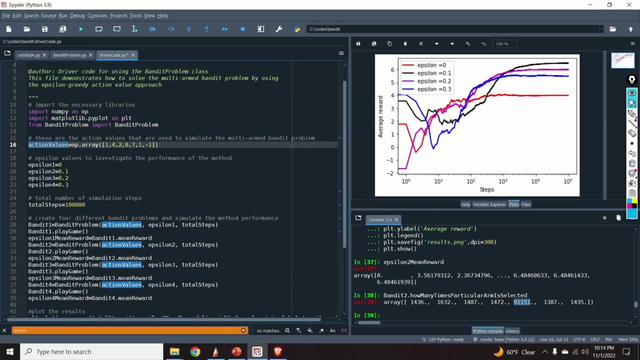 run the algorithm, obtain mean rewards and then repeat this many times and compute the average of the mean rewards to obtain a good insight into the statistical properties of the algorithm. okay, that would be all for today. I hope that you like this video. if you like the, 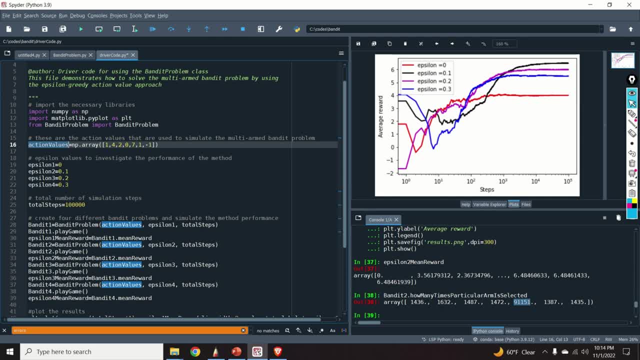 videos I create. please subscribe and support my channel. thank you very much and have a nice day. 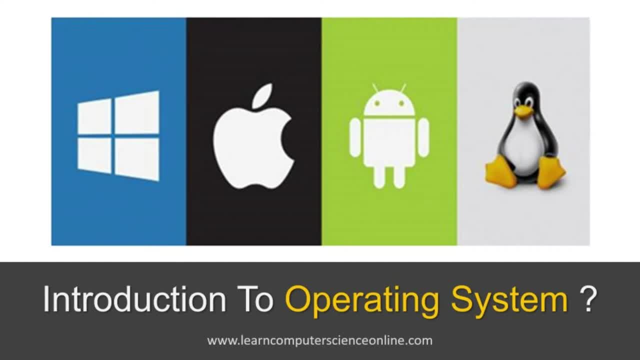 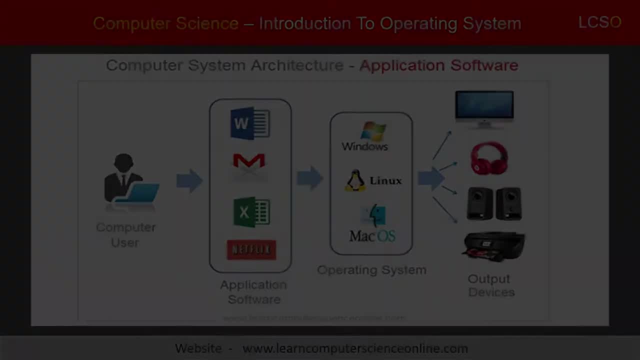 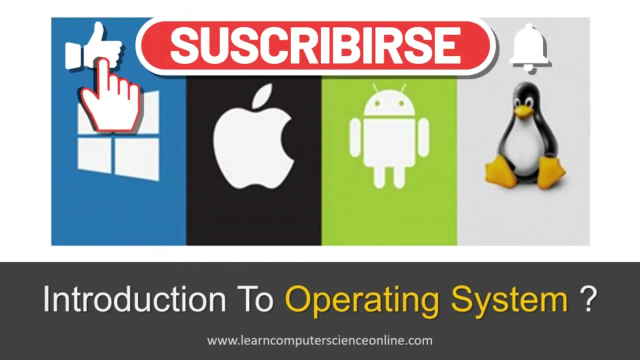 Welcome to learncomputerscienceonlinecom, and in this video we are going to discuss what is an operating system, its functions, types and its importance in computer architecture and organization. Let us start with a simple, brief introduction to the operating system.